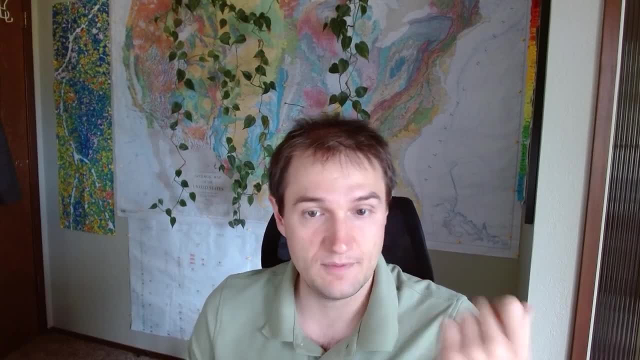 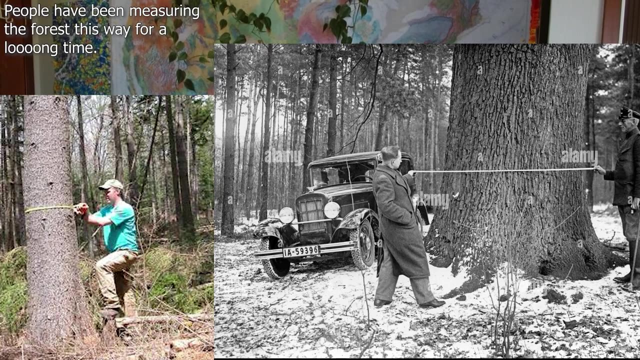 that area. What are we measuring? We're usually measuring diameter, So diameter at breast height, which is basically how how wide the tree is at 1.3 meters off the ground. It's very easy to wrap a tape measure around a tree from that height. 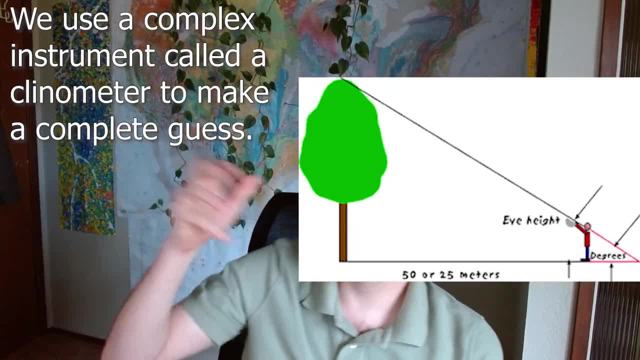 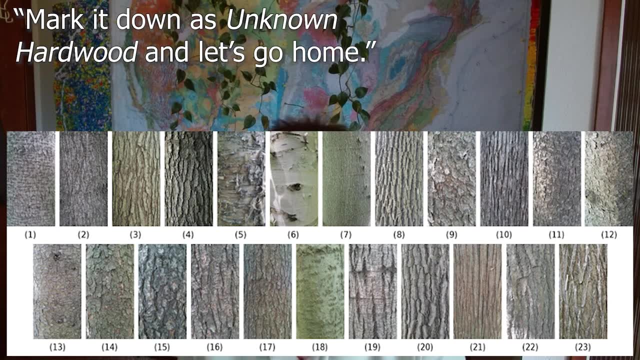 We're measuring height of the tree usually, So we usually use like a clinometer, which is a measuring instrument, to measure height, And then we measure species. And using those three things we can use a set of equations called allometric equations. 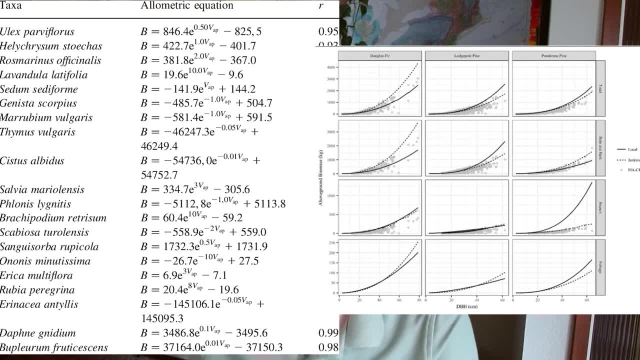 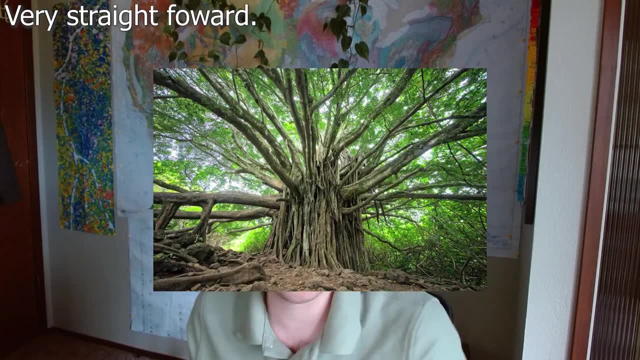 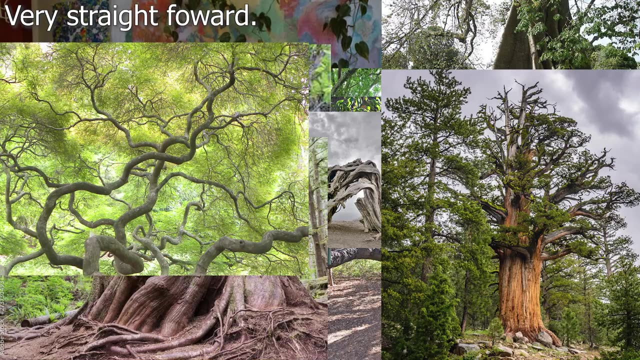 That basically correlate the diameter and the height and the species with the amount of carbon in the forest. So we can say, for example, with an allometric equation: you know a species, you know this particular species of tree of this diameter and of this height has this much biomass? Now, I quite frequently 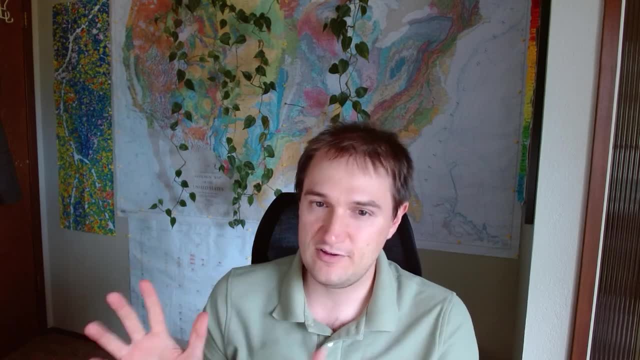 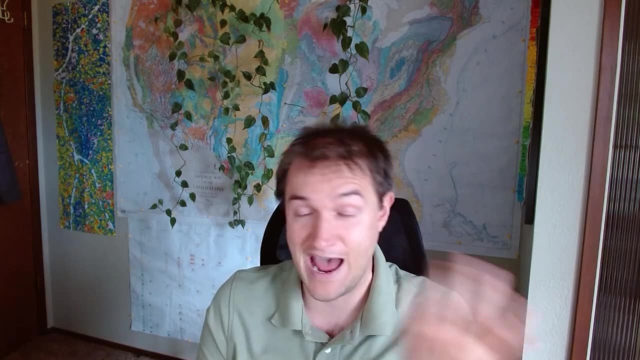 say the term biomass and carbon, and that's because the two are basically the same thing. I mean, biomass just refers to the weight of the tree, but carbon is a basically half of biomass. So the two are basically the same thing. So we're. 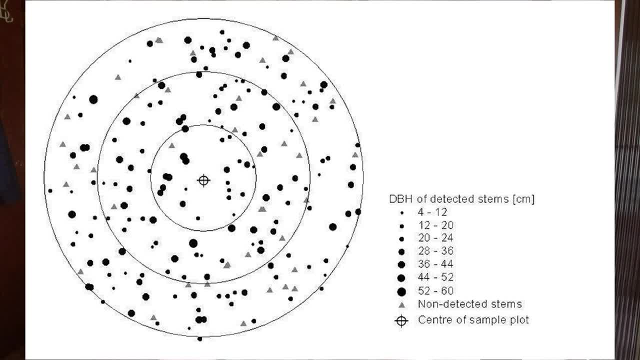 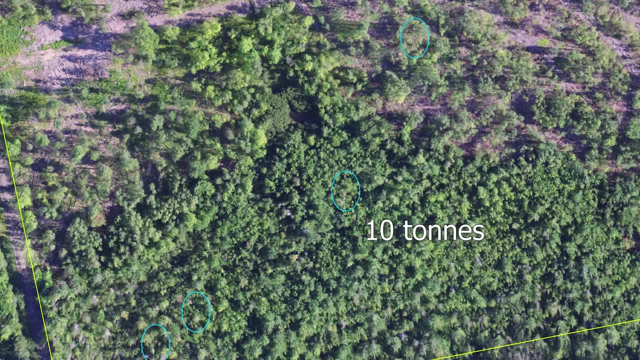 measuring carbon on all the trees inside of our plot. So what do you do with that? Well, you sum it up and you get a total amount of carbon inside that plot. Now the plot is, let's remember, it's a tenth of a hectare, right? So if you wanted to, 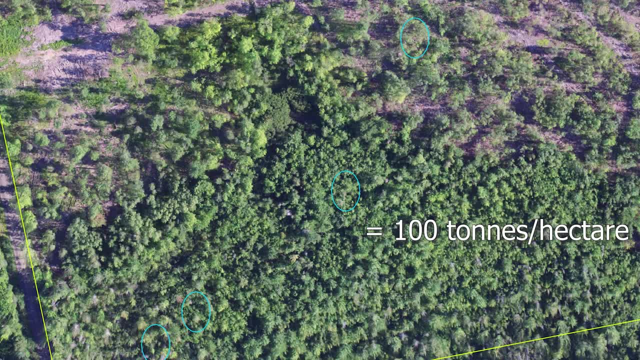 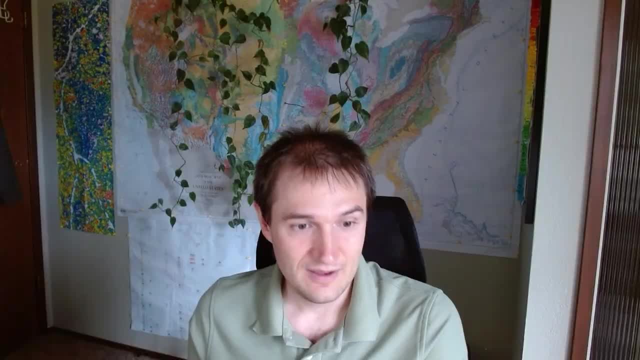 know how much carbon there is per hectare. you know in that plot. you take your sum of all the carbon that you've measured in your trees and you multiply by ten and that gives you a per hectare value. Now remember, you've got a hundred. 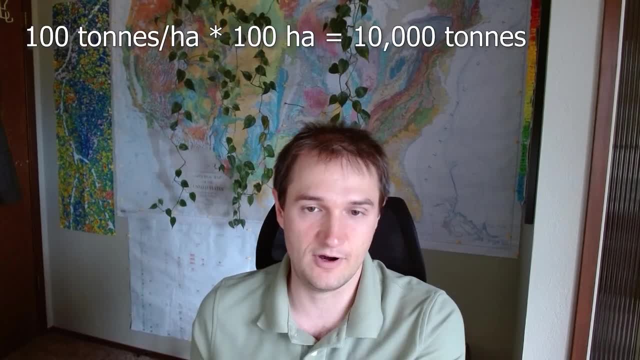 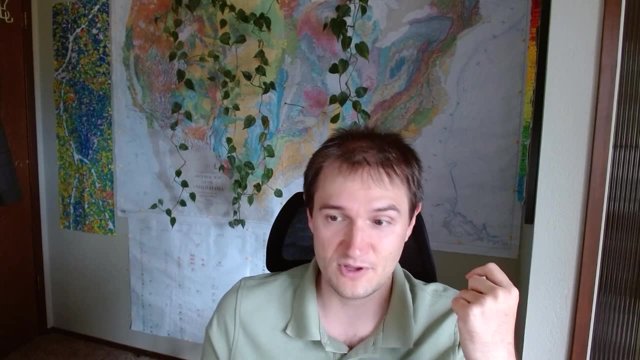 hectares. so you multiply again by a hundred, and that's how much carbon you have on your, on your landscape. Alright, so that's all well and good, but you've only measured one plot, one pretty small plot. So how do you really know that this? 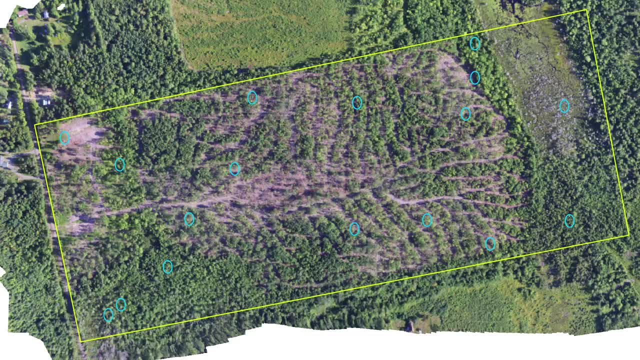 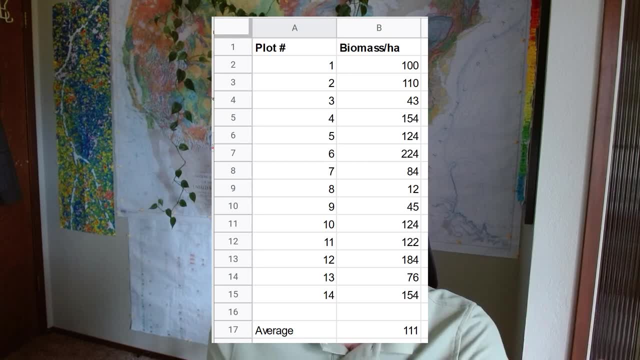 is the right measurement. Well, of course you have to measure a bunch of plots and you measure, I don't know, let's say, 50 plots inside your little area. You then basically take the average biomass per hectare from all. 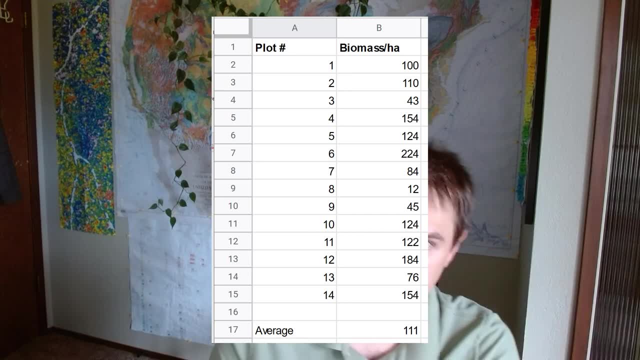 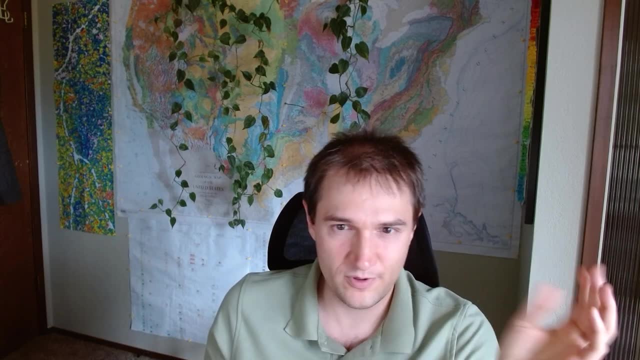 50 of those plots. Now, some of them are going to be low, so maybe 80, and some of them are going to be high, maybe 200. So how do you know which plots are actually, you know, representative of your forest right, Because you've got this range. Well, 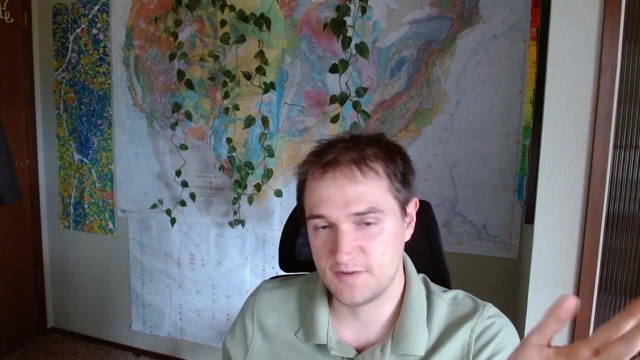 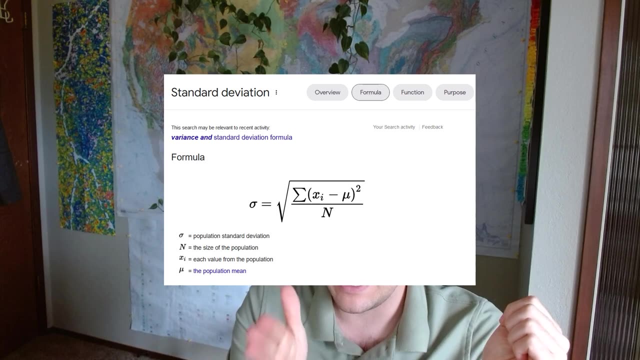 here's where we can use some basic statistics, Because we have measured something like 50 plots. we actually know the variance of the measurements that we've taken and our goal here is to figure out what the mean is And what we can basically do is reconstruct a distribution. We can reconstruct a bell. 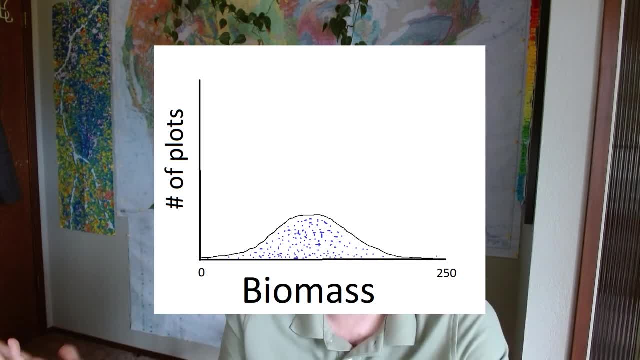 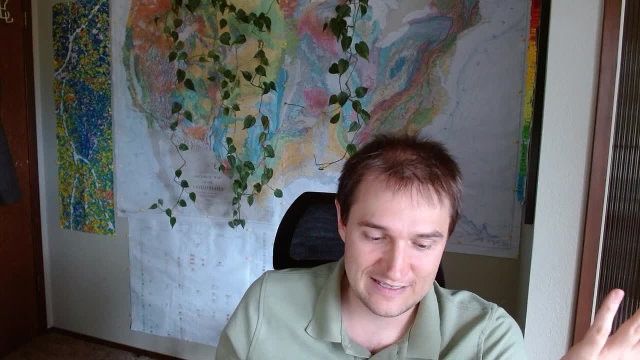 curve that corresponds with the biomass in the forest and the middle of the bell curve is the average biomass. and that's what we're trying to figure out Now. with these basic statistics, we can basically say, because we've measured 50 plots, the 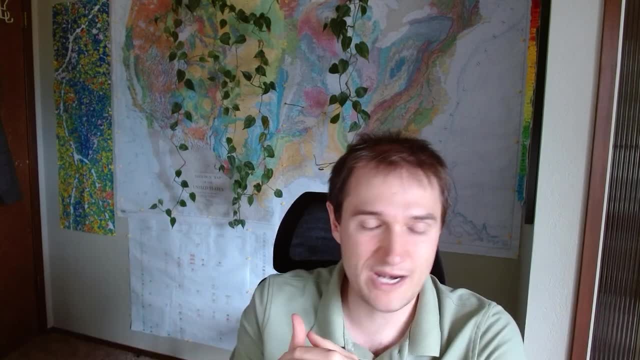 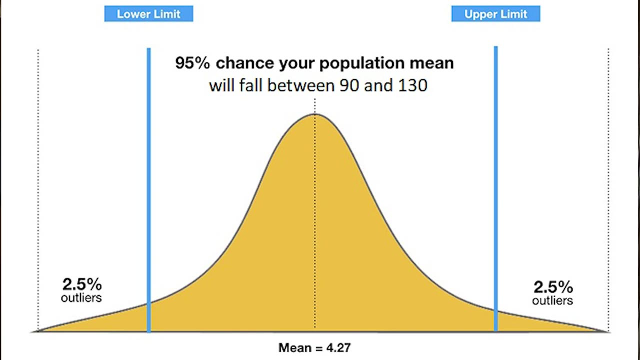 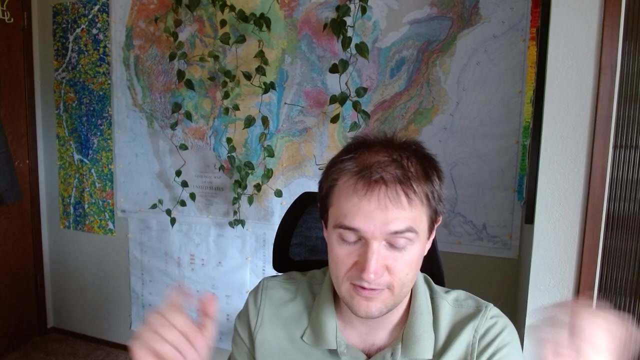 variance of the plots is, let's say I don't know, 20%, and then we can use that to basically calculate a confidence interval and then say this is our average and plus or minus, I don't know. let's say 5 tons at 95% confidence. So we can measure this confidence. 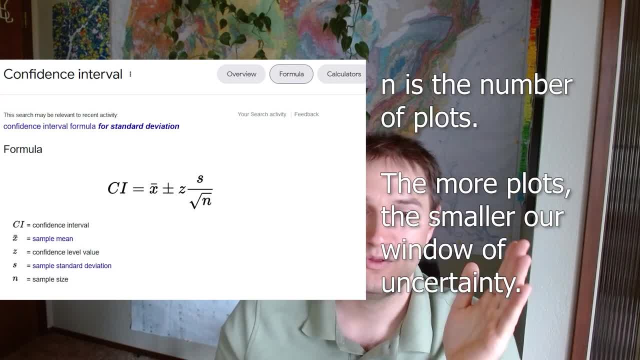 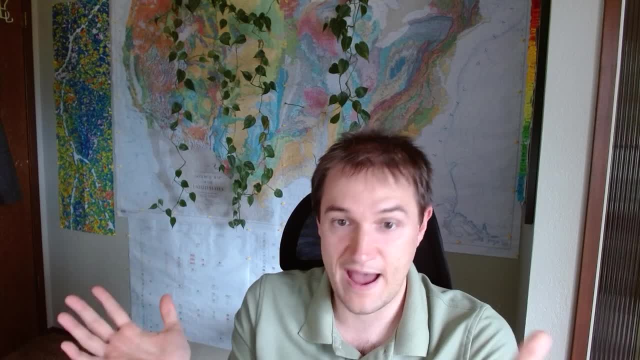 interval and, essentially, the more plots you measure, the more confidence you have. So, the more plots you measure, the closer your average is going to be to the actual answer. and, in fact, if you were to measure your entire forest, if you were- 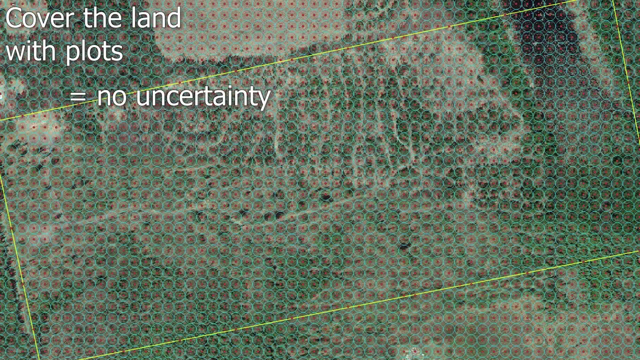 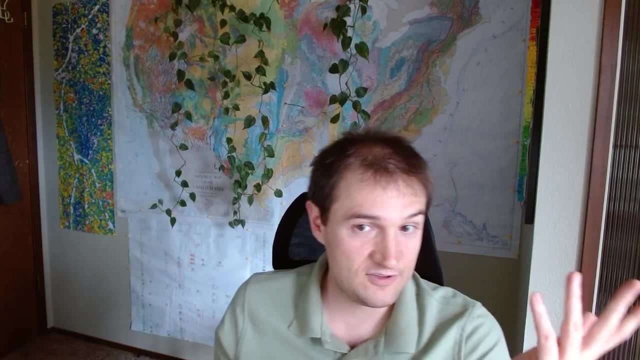 to measure just a series of plots that cover your entire land, then you would have no error at all. right, You've measured every tree and your average is right. That is the actual average. So we don't necessarily want to do this, We want to measure. 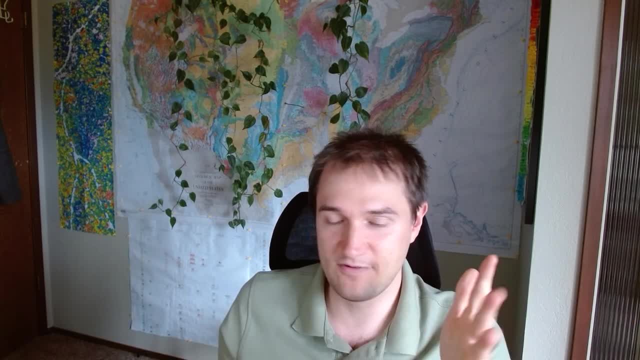 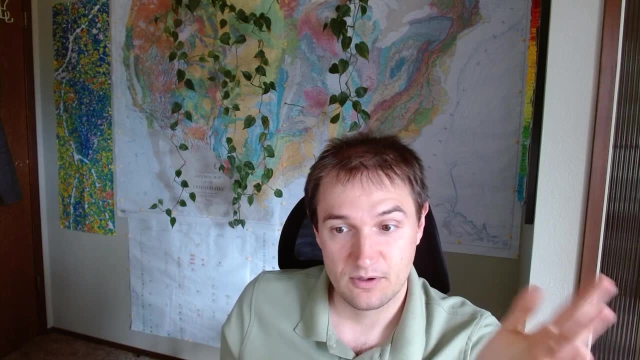 some number of trees that gets us close to that average, but we never actually want to measure every single tree. So the more plots that we measure, the more confident that we are about our average. And so we measure more and more plots until our confidence interval decreases to a point. 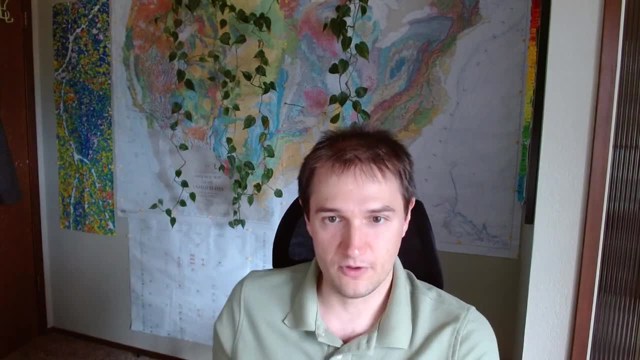 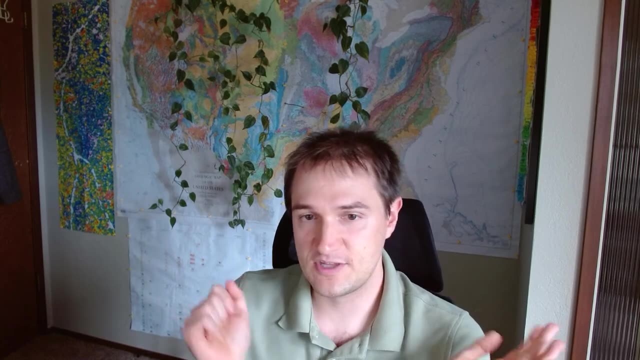 in which we're satisfied. Now, most carbon protocols have some level of confidence interval that you have to measure your plots to. So a lot of the time it's plus or minus 10%. That means that you measure a bunch of plots, you have a mean, you have a variance and you compute your. 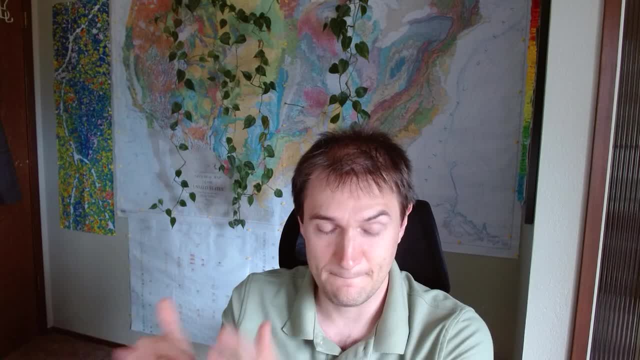 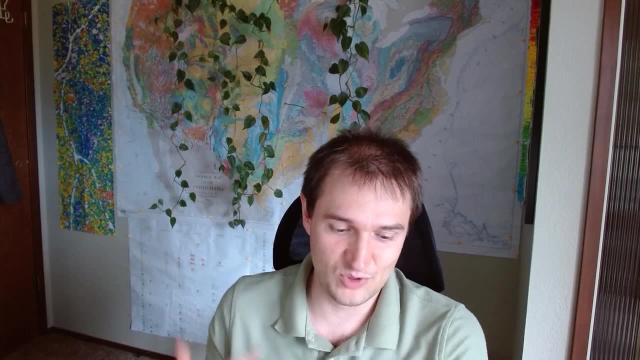 confidence interval, and that confidence interval is plus or minus 10% of your mean. So how do you know how many plots to measure? How does this actually come about? Well, I mean, basically, what we're doing is we're measuring plots until we reach the confidence interval that we want, And 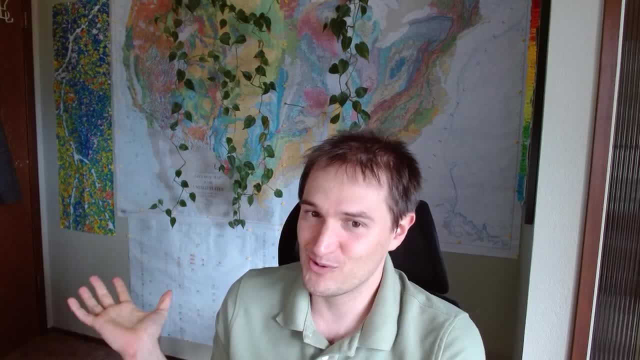 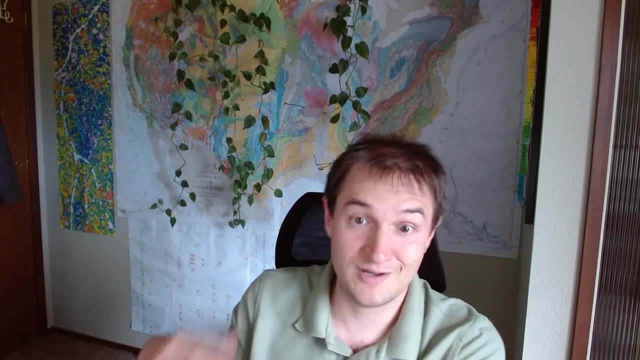 that's not a statistically sound way of putting it, but that's basically what we're all doing. We're basically we're going out there. maybe we measure 20 plots. we get a confidence interval of 15%. Okay, we got to go measure another five, And then we get a confidence interval of 7%. All right, 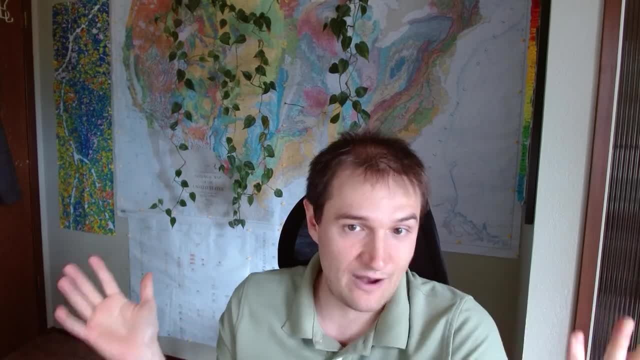 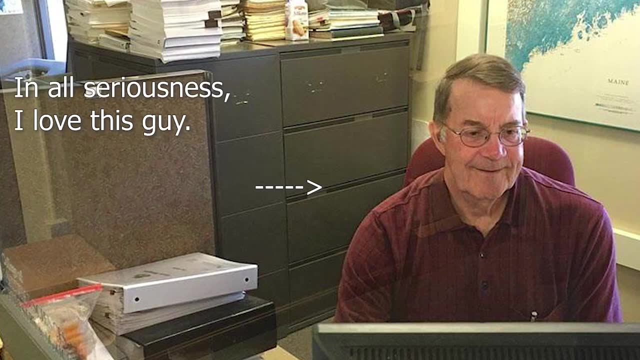 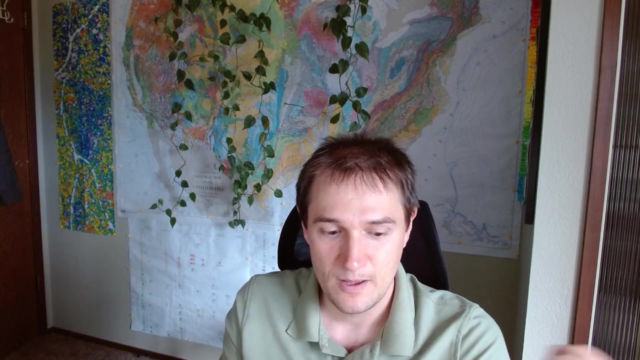 we're golden, And so that is how we create an inventory for forest carbon, And that's a pretty good way of doing it, because it's got a lot of statistical certainty to it. We know that trees fall along a bell curve, just like every other biological mechanism. We just 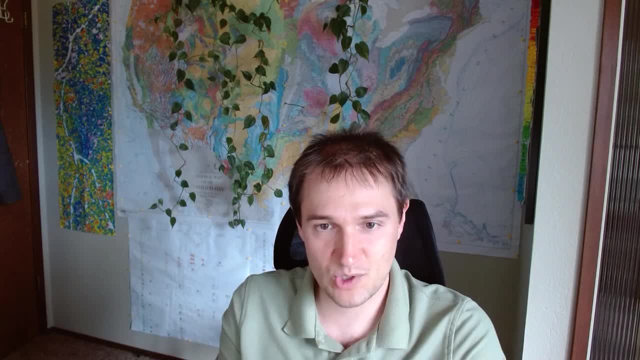 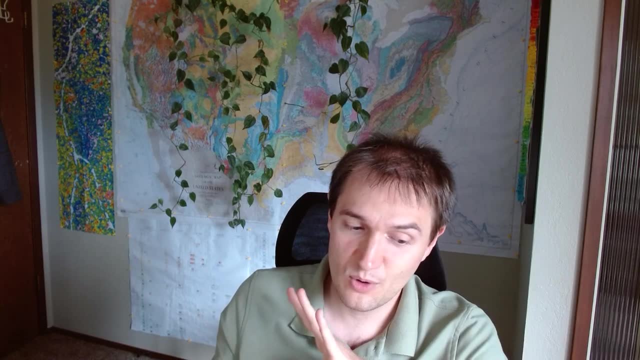 need to measure a confidence interval of 15%, And that's a pretty good way of doing it, because we need to quantify what that bell curve is. If we measure more trees, we get more accurate. It's very nice, The statistics are very nice. So that's the high level overview, And you can stop watching. 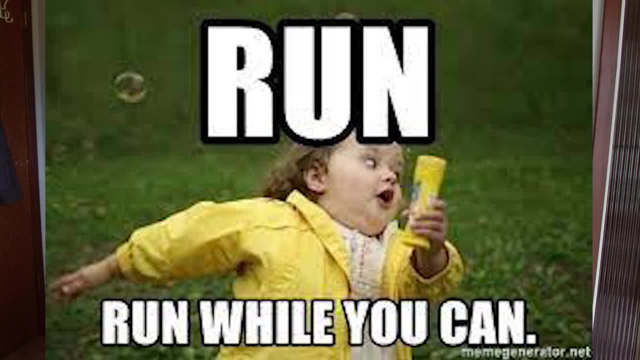 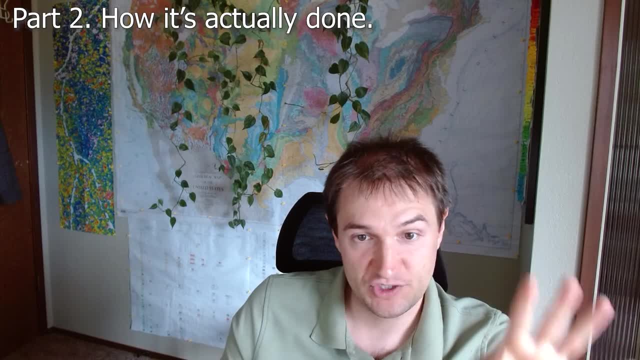 here, unless we want to dig in deeper. And boy are we going to dig in deeper. So one of the problems that we have to face with the scenario that I just drew out, where we've got 100 hectares and we're going to measure something like 20 plots or whatever it is, 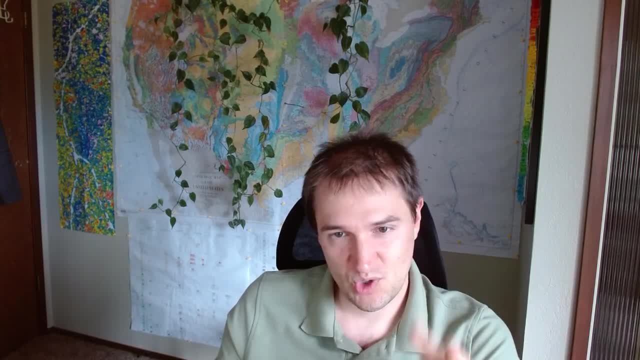 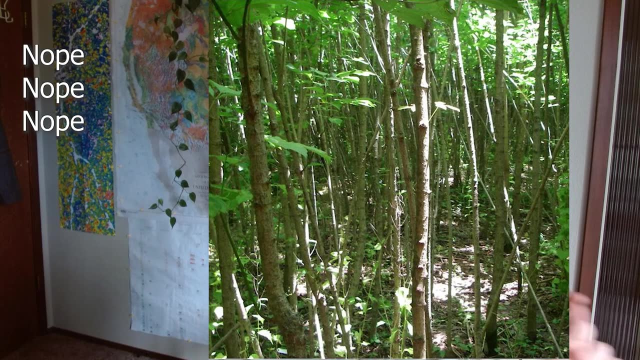 is that we really don't want to measure every tree inside those plots, And especially we really don't want to measure all the little trees, because there are so many little trees- I mean, when trees are small they pack in really tight, And so you could end up measuring thousands. 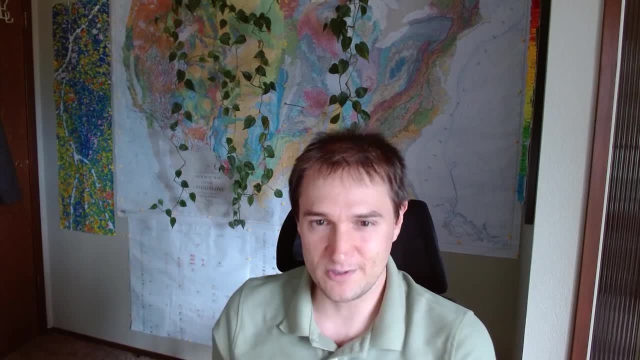 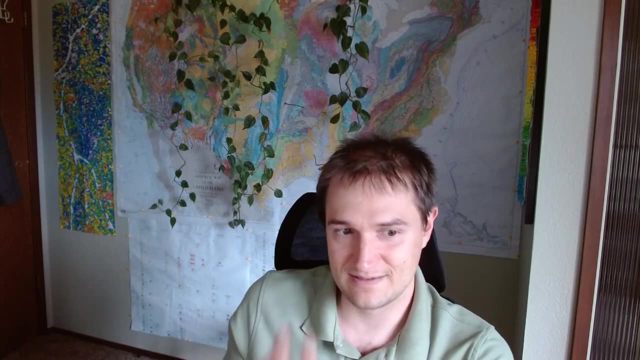 of trees on each one of your plots, And so what's an easy solution to this? Well, little trees make up less carbon, So we really don't need to measure as many of them. We don't need to measure them as confidently as we did before, And so we don't want to measure every tree inside those plots. 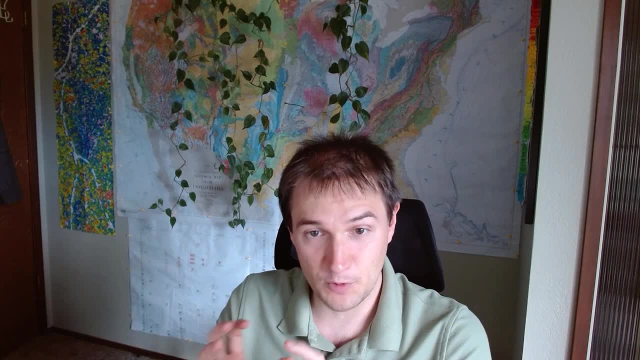 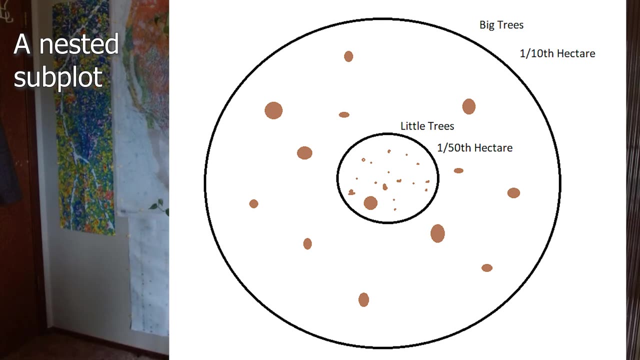 What we can do for the little trees is we can just have a smaller plot, And so we've got our 10th of a hectare plot in which we're measuring all the big trees. Maybe we want a 50th of a hectare plot in which we measure all the little trees. Well, I mean, that's fine, You just have. 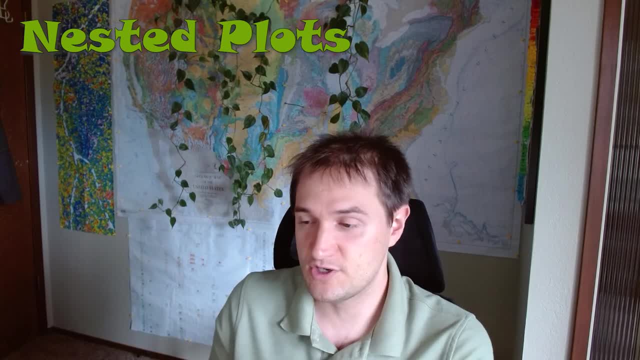 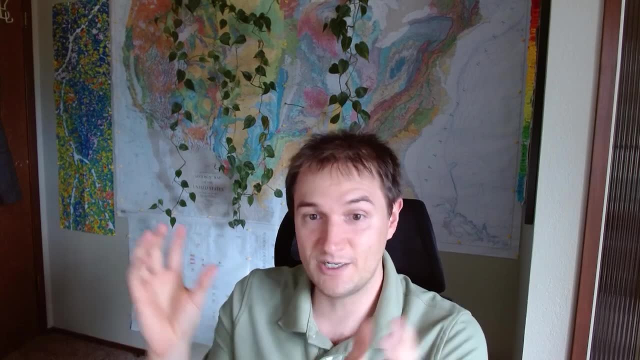 to use a different expansion factor. right, So you're going to sum up all your carbon inside your big plot. multiply that by 10.. You're going to sum up all your carbon from your little trees inside your little plot. multiply that by 50, add the two together and that's your. 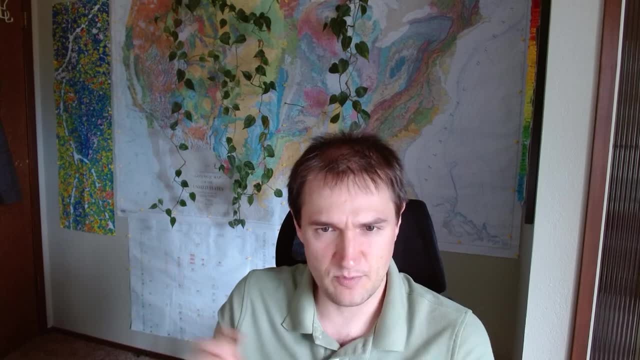 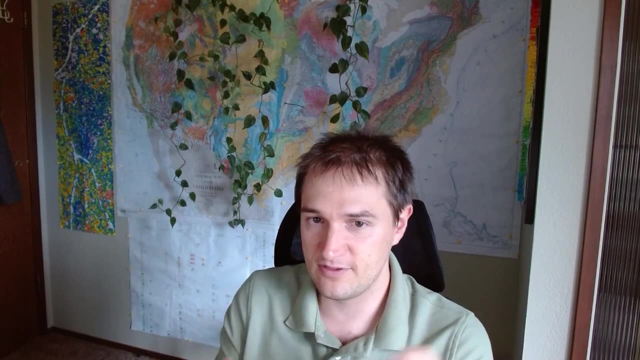 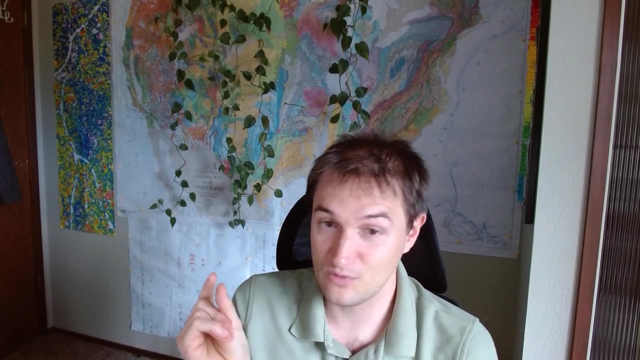 per hectare carbon value right. So now we're nesting plots. Now, people don't just do this with little trees and big trees, They nest plots, you know, with different sizes, Because you know, if we're talking about trees that are this big, even a 50th of a hectare may be too much. I mean. 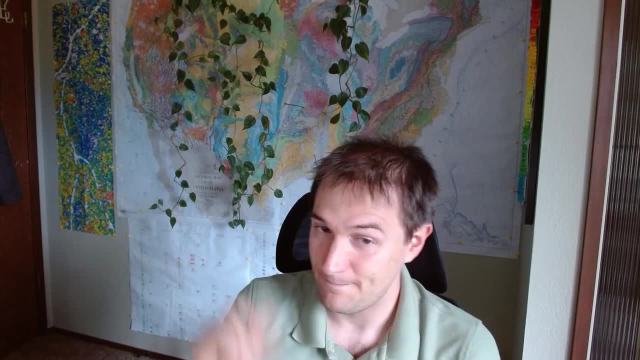 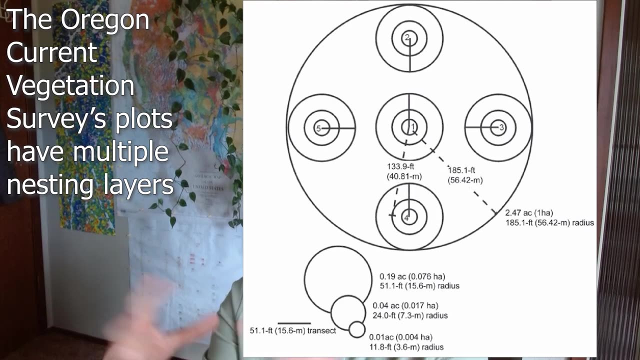 we could be spent an entire day measuring trees that are this big, And so you know, maybe we have a really small plot for really teeny saplings, Maybe we have a medium-sized plot for like medium-sized trees and a bigger plot for big trees, And so you know a lot of these plots. 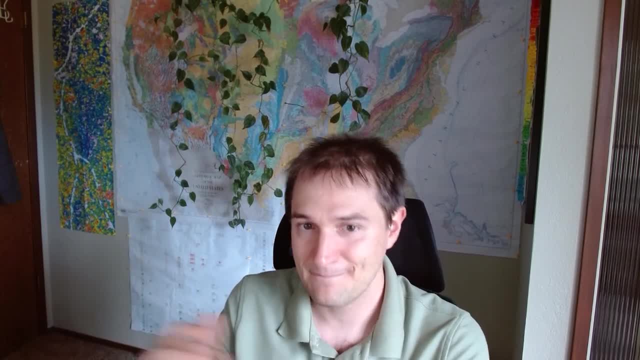 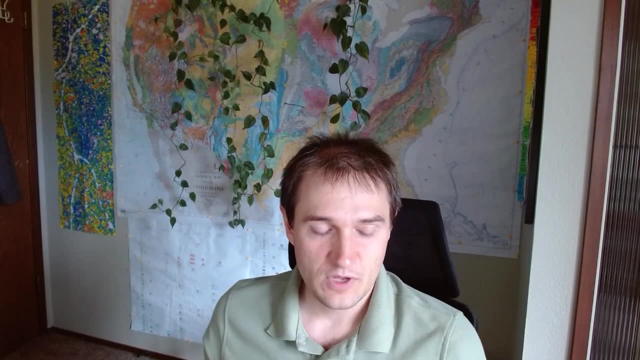 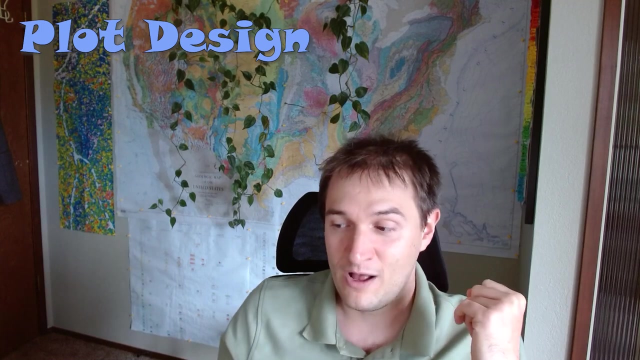 are kind of like nested dolls And you can keep track of them, and that's okay. This led to a different type of plot design. So you know, as you may be intuiting here, plot designs are not always that straightforward, Because, well, frankly, every scientist out there thinks that. 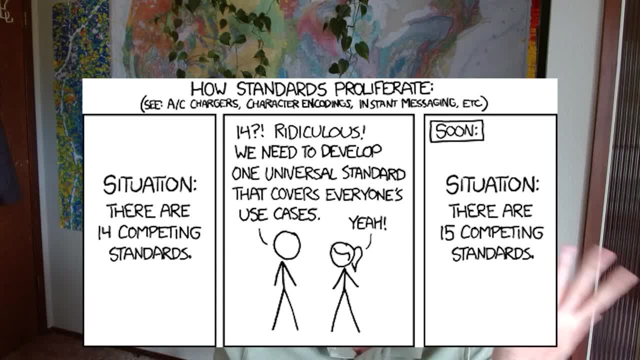 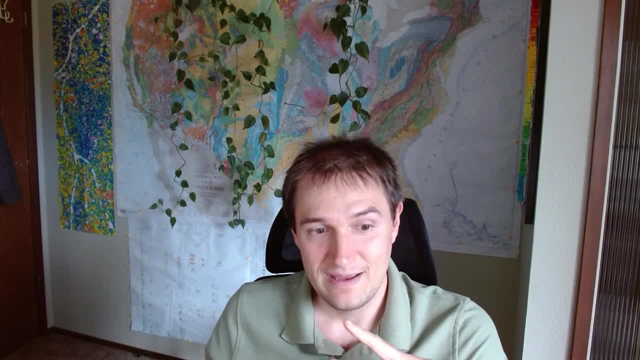 they're a smartass and thinks that they've come up with a better way of measuring the trees, And so there are hundreds of different plot designs that exist out there. Another thing that people do is they will measure plots in a series of subplots, And so, for example, the US Forest Service. 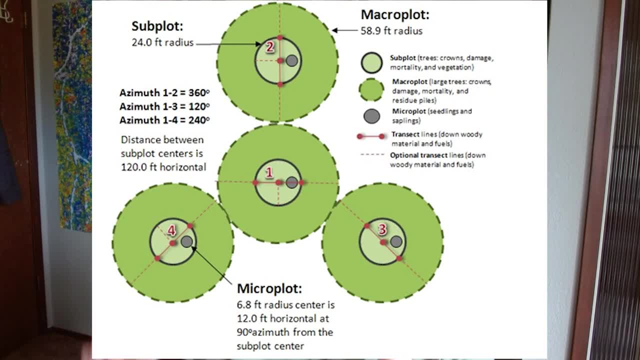 National Inventory does what's called the turkey foot method, where they have a series of subplots that are placed in like a turkey foot pattern And then within each of those plots there's even smaller plots where they measure all their little trees. That sounds kind of dumb, dumb, dumb. 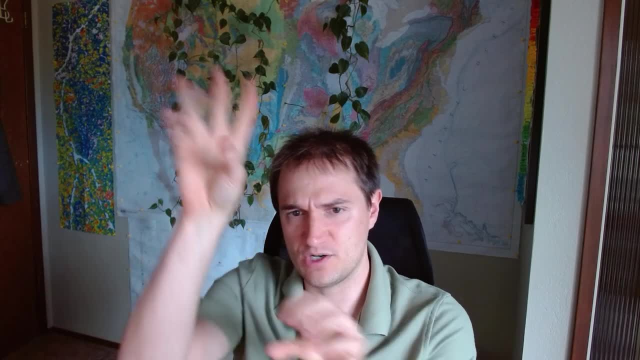 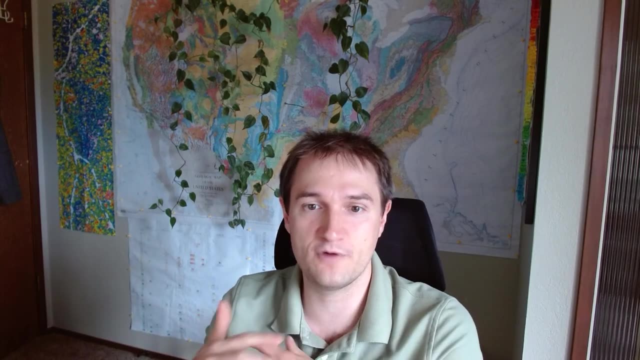 dumb dumb. Now why do they do this? Why don't they spread out a bunch of little plots instead of just doing one big area? It's a stupid idea, to be clear. But they do it so that they can capture more variety, So that they can say: you know, they have a larger. 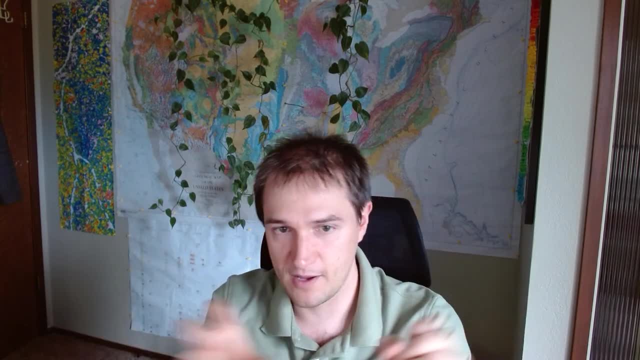 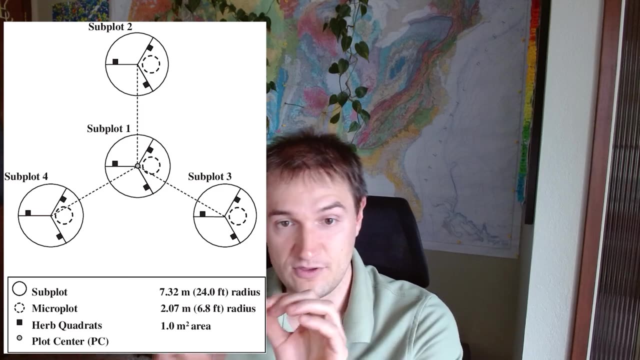 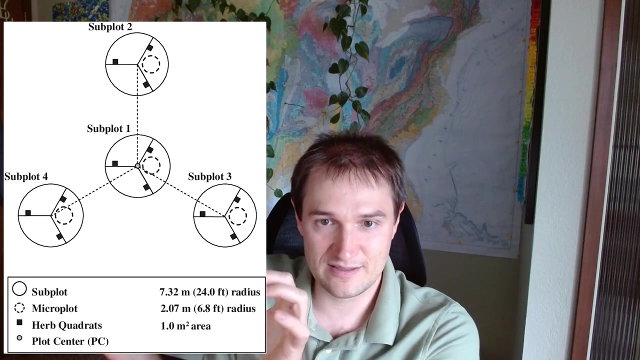 chance of that subplot falling within a clear cut or something. The reason it's a stupid idea is because you lose GPS accuracy for one. So I mean the odds of you like being able to correctly track 120 meters out on an azimuth of 60 degrees and properly end up where your 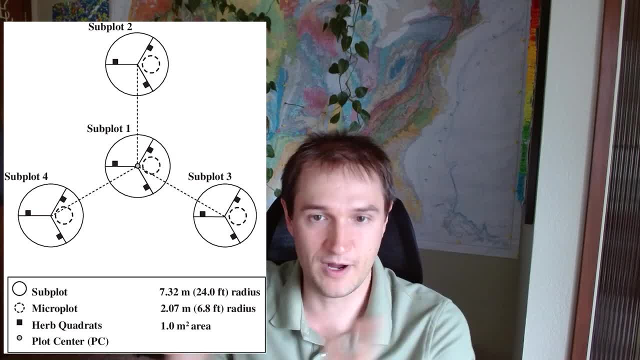 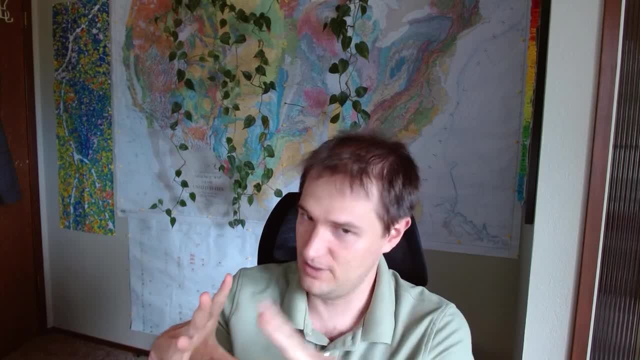 subplot is that's not so great. So your subplots are going to end up all kinds of funky And you, you know you also, you're just. you end up taking these really tiny little microplots that don't do anybody really much any good. So this is, this is a mistake that a lot of people make, but they're. 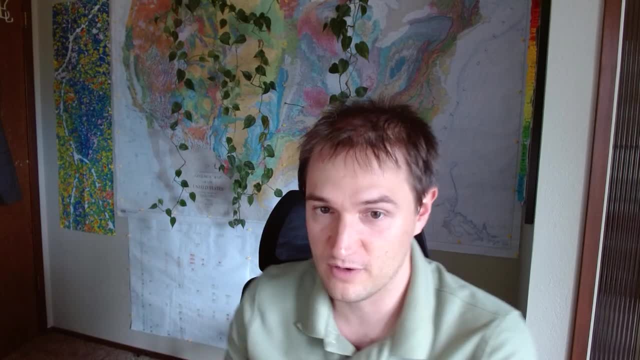 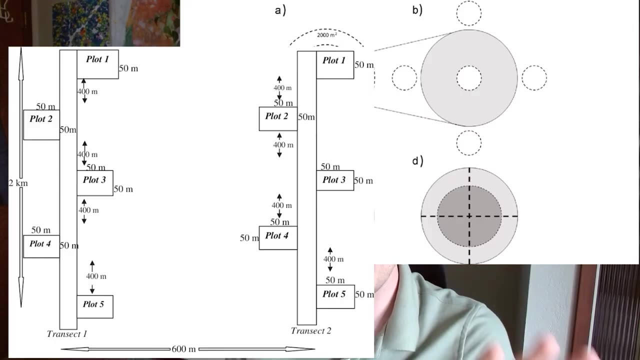 making this mistake because they think that this is, you know, capturing more variety on the landscape. Every type of possible plot configuration that you could ever imagine I have seen. I have seen plots that look like they're alien spaceships. I have seen plots that look like they're. 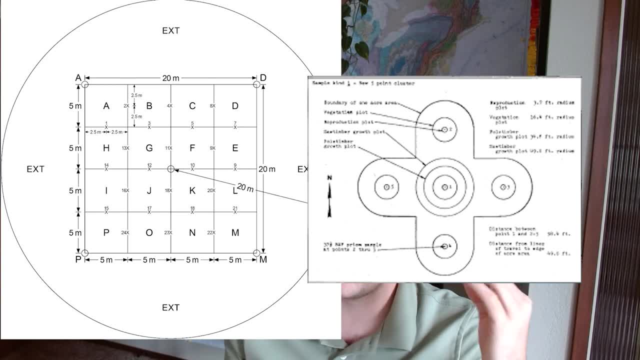 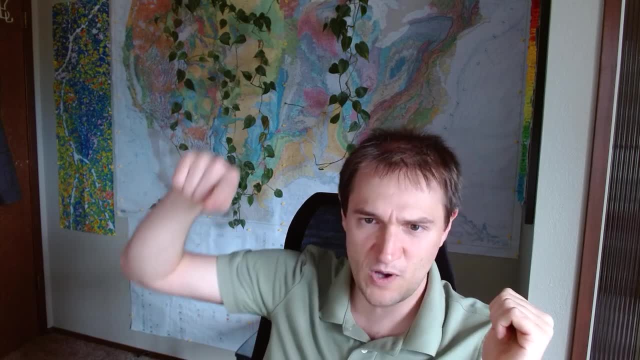 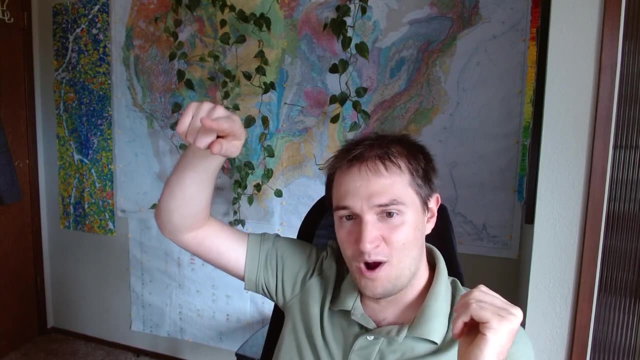 plot circles. I have seen plot configurations in which they're walking in a straight line, measuring every tree on five meter sides, and then, if you hit a big enough boulder, you are to bounce off that boulder like like the refraction index of a of a light ray, and then start walking in another. 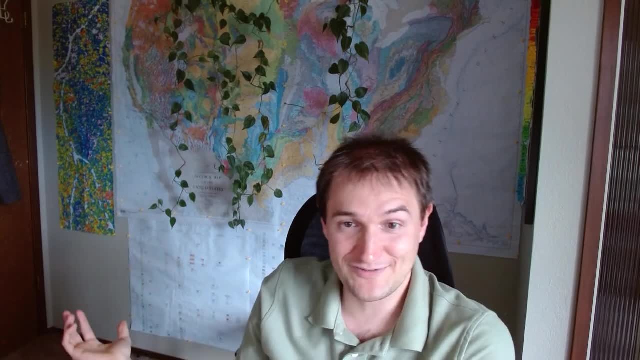 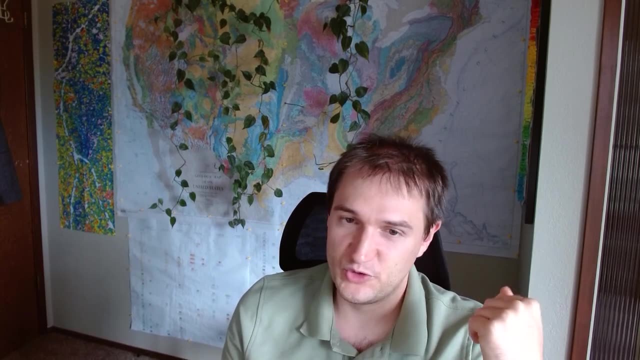 line in another direction. Like this is the kind of absurdity that I've come across on plot measurements. So that's out there, And every- you know, every- National Forest Inventory has their own plot network And it's it's a genuine nightmare to try to, to, to patch all these. 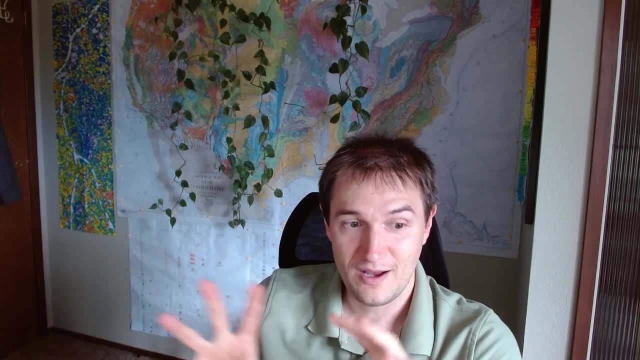 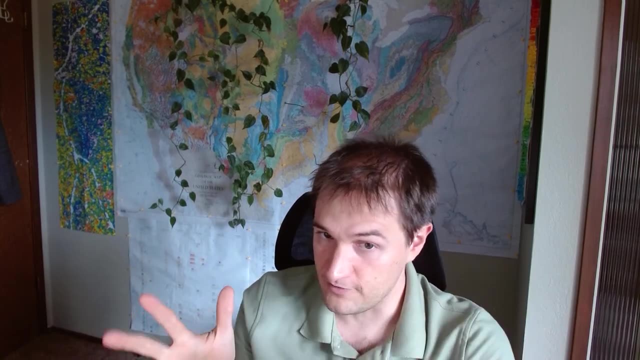 different plot networks together and create a cohesive network for actually, like training, a remote sensing model. Okay, So, so that covers complicated plot designs. However, there is a different type of design out there, called a variable radius plot, And the way that this 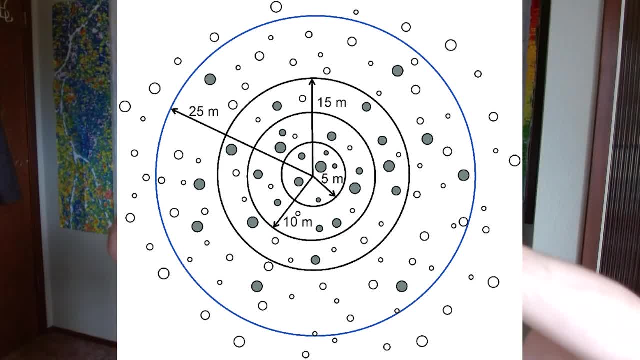 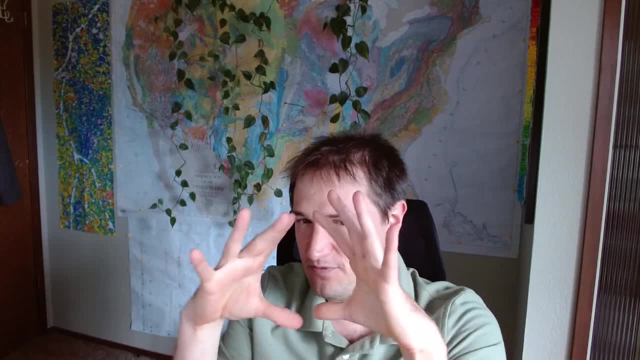 works is that, instead of doing, let's say, three concentric nests where you're measuring really teeny trees and then medium-sized trees and then big trees, the idea is is that you, you can do an infinite number of nested plots, And what I mean by that is that maybe for an 11, 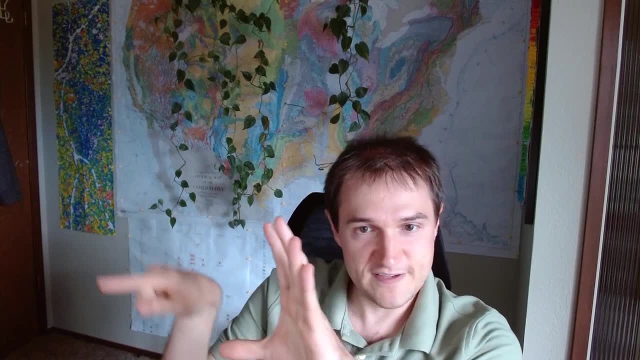 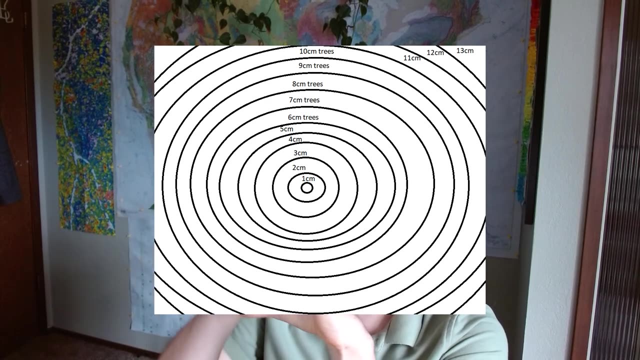 centimeter wide tree, there's a circle in which all the 11 centimeter wide trees would fit into, And for a 12 centimeter tree, there's a slightly bigger circle in which all the the 12 centimeter trees would fit into, And you basically do this into infinity, so that if you're dealing with a 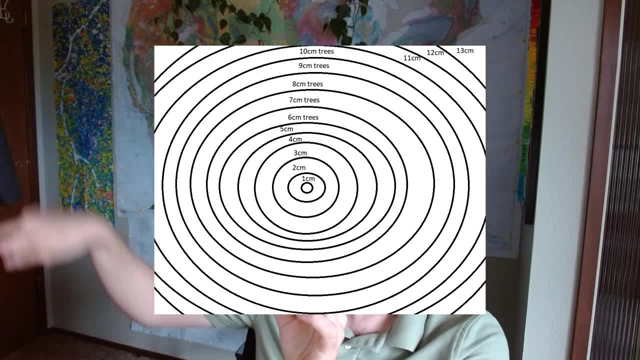 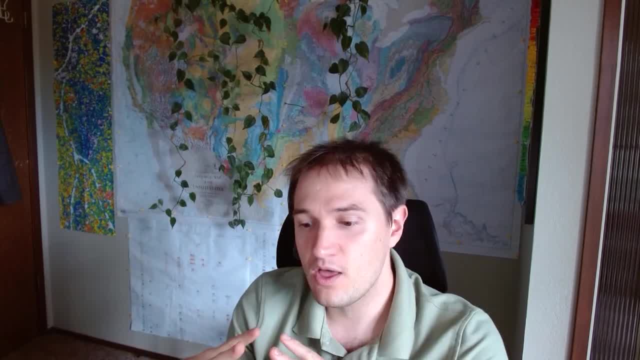 really, really big tree. you've got a massive area in which that could fall in inside the the plot that you're measuring. Why on earth would you do this? Why would you make this more complicated? Well, the answer is: 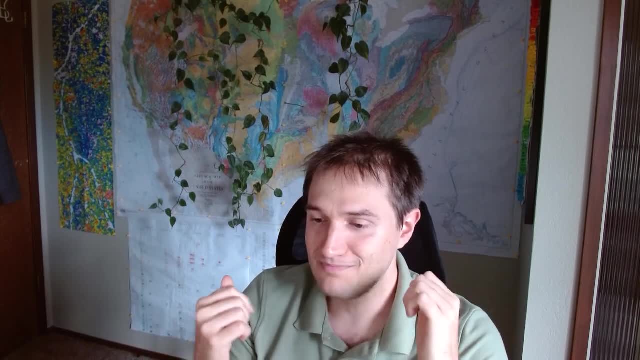 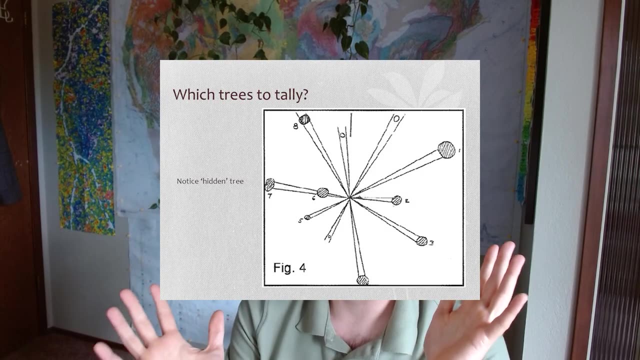 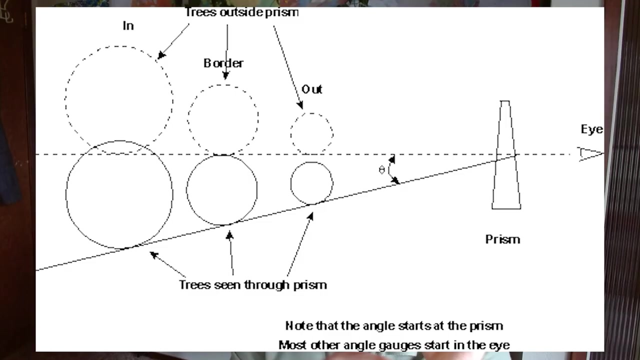 is because you can use basically a trick of trigonometry to measure these variable radius plots very quickly. And the way that you can do that is you can basically use a, uh a a prism that's basically refracting light- uh to basically see which which trees would be inside those plots. 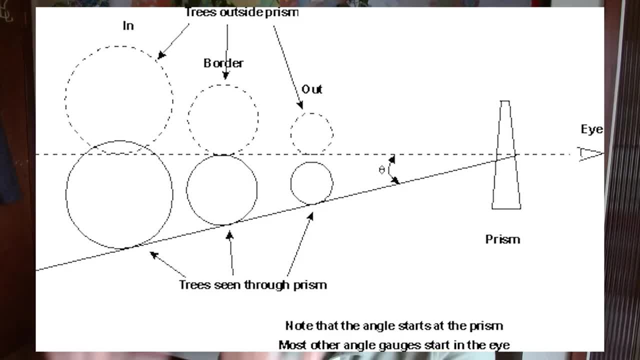 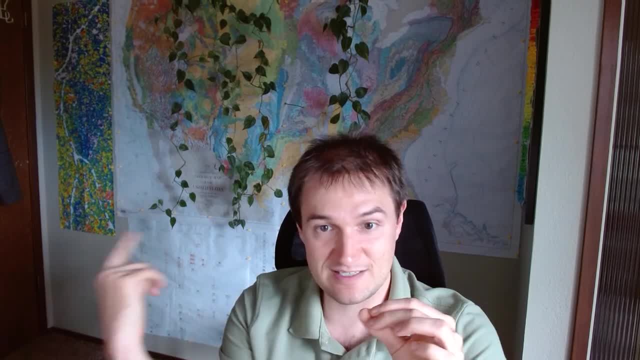 and which trees would be outside those plots. Now, this is very, this is very exciting and very sexy if you are doing field inventories, because, uh, it is really difficult to go and measure the distance that every tree is from a plot center. 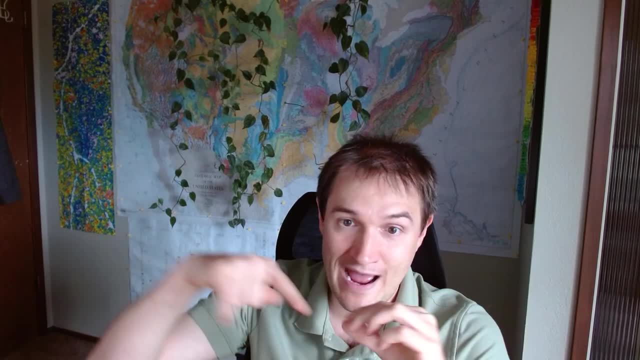 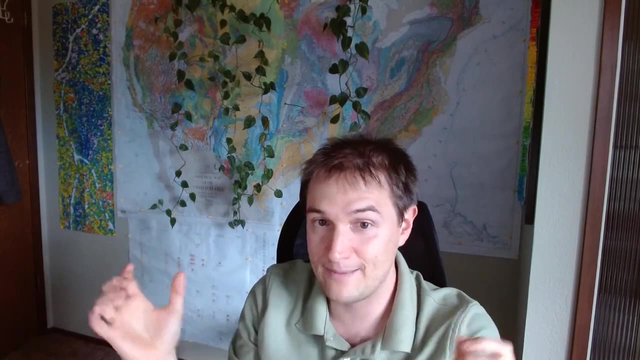 right. So in our, in our standard approach, we have to plot out something like a 13 meter distance and then we have to see if every single tree is within that 13 meters. And we have to do that maybe three or four times for for each concentric plot size. It takes a long time. You have to measure. 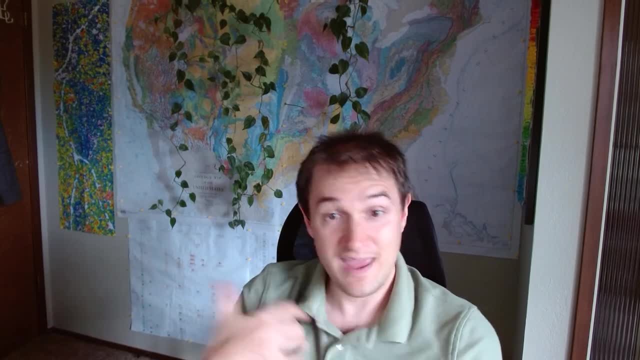 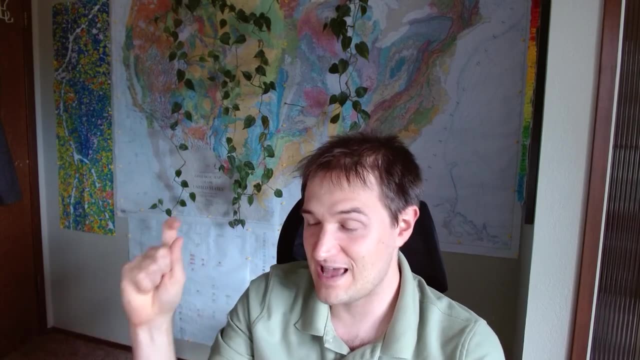 the distance of pretty much like every tree that might be on the edge. But here we have a solution that basically uses a trick of geometry, where you can just stand at the plot center and just swing a prism around and say, uh okay, this tree's in, this tree's out, this tree's in. 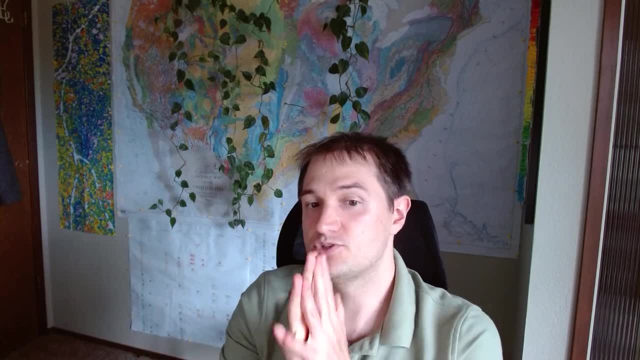 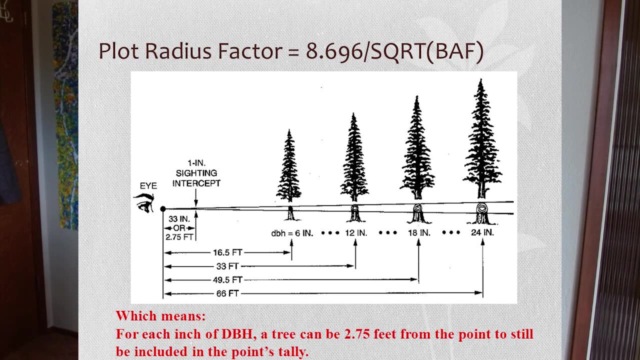 this tree's out and then go and measure them really quick And it's very easy. So that's great, Uh, and? and so people use these variable radius, infinitely nested plots, uh, to make measurements of the forest. And there's nothing wrong with that, They're. 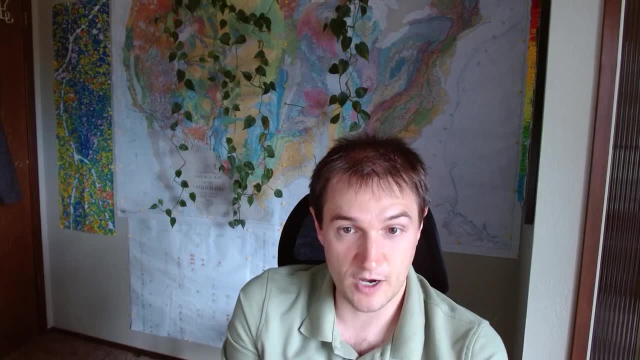 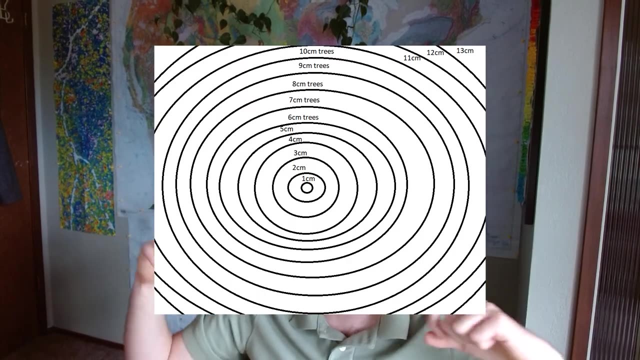 they're perfectly good at making statistically valid estimates of of carbon. right? It's the same principle. It's just that there's an infinite number of of of nested sizes. If you had a tree that was like size of Mount Everest, you would be able to measure it. if your plot were on the moon. 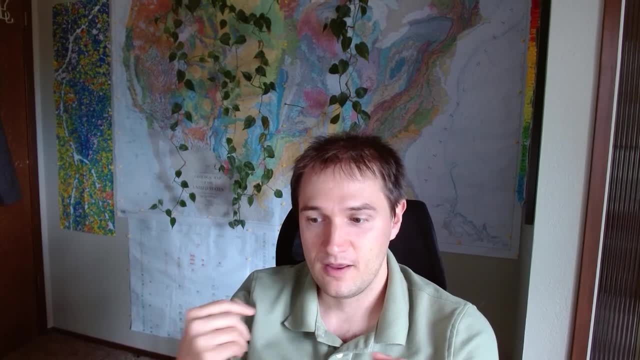 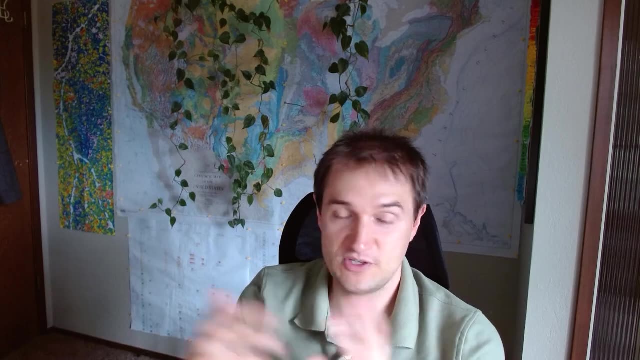 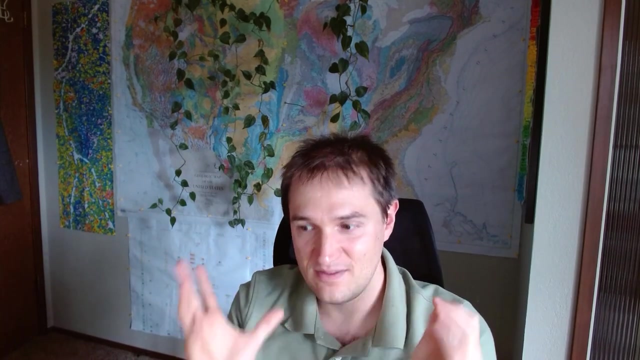 Okay. So what is the implication there? Variable radius plots are really quick to take. You can take like two or three times as many of them. Um, they're still statistically valid, but there isn't actually an area that you can look back to and say: this is where I measured the trees. 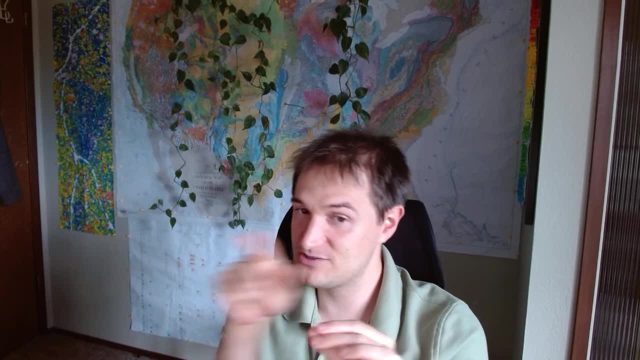 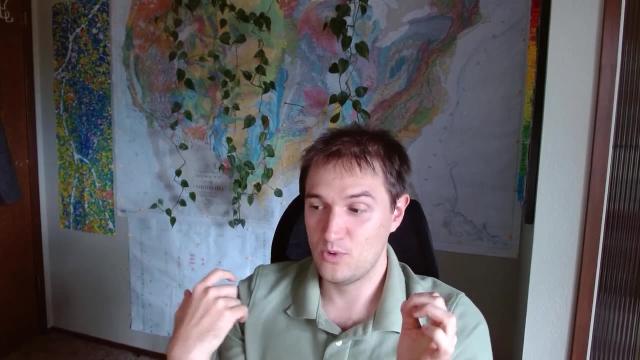 Because, you know, there's a different area for every, for every tree that's a different size, And so, uh, this becomes really difficult if you're trying to pair it up with remote sensing data, because, uh, we like to be able to basically say: this is how much carbon there is in this. 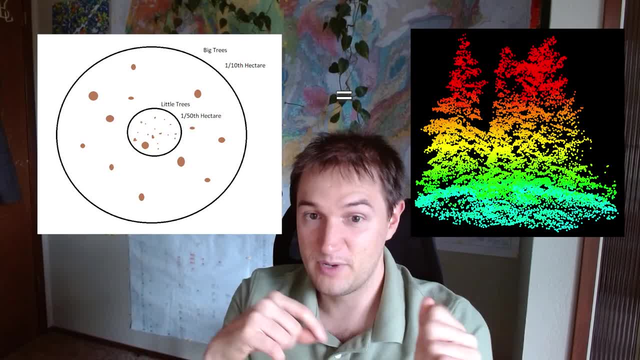 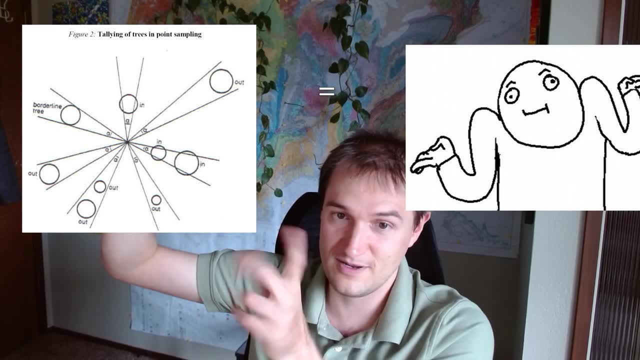 little area And this is the remote sensing data for this little area but for a variable radius plot. you basically just have a point and you know the trees could be measured, you know anywhere from who knows how far away from that point. 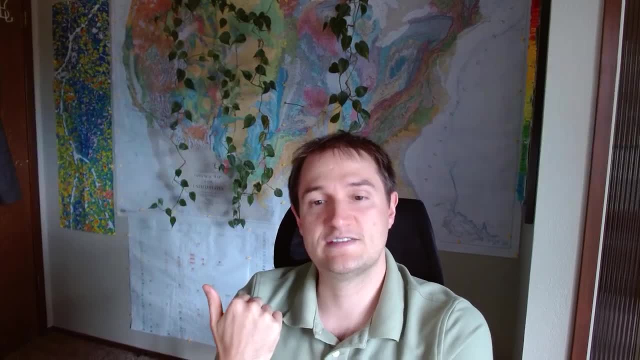 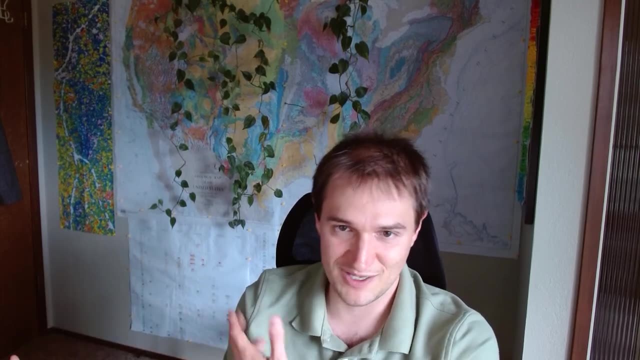 Um, and so that makes it much more difficult to work with remote sensing data. you can still kind of do it, but it's definitely less accurate and you need more plots And and of fierce debate out there about the level of accuracy that you can get if you're using. 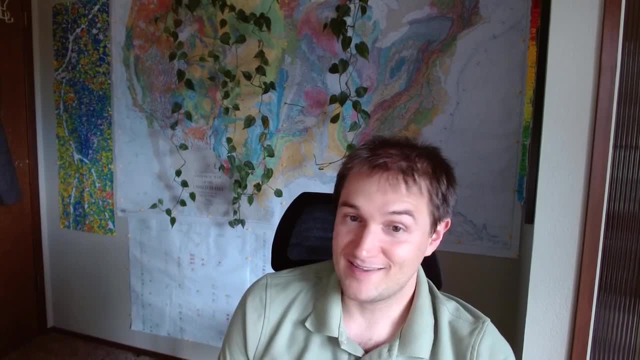 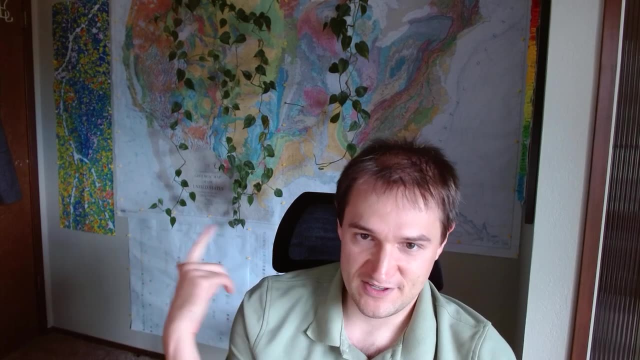 variable radius plots that don't actually have edges. Believe me when I say it's difficult for everyone to grasp this concept. Another way of thinking about it is that every tree has associated with it a circle in which you know that tree's measurement would be valid inside. 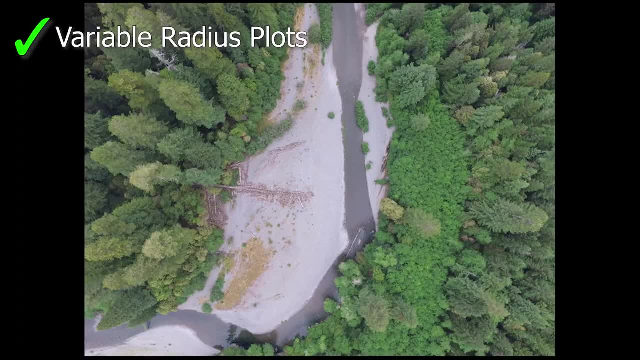 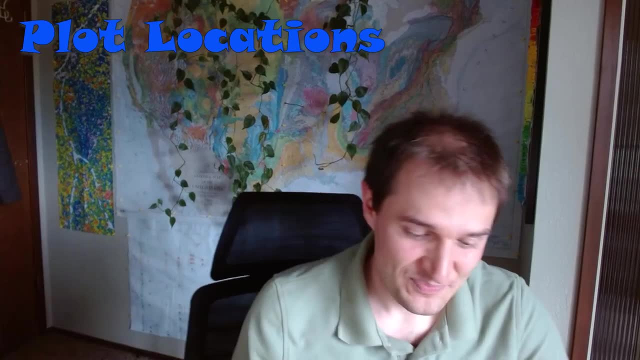 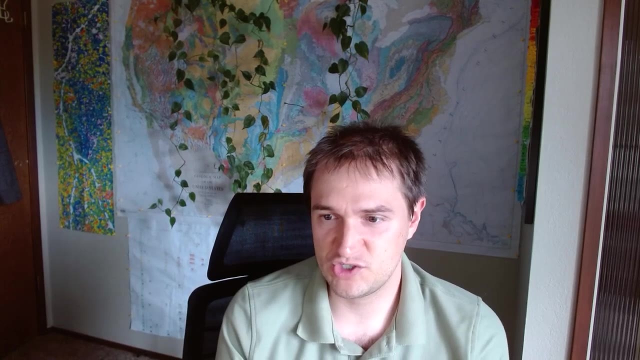 you know we're not going to touch this. Forget it, Forget it, We're moving on. Another big issue with forest inventory plots is the GPS precision. Now, this doesn't matter too much if you're just trying to measure like a huge area, like 100 hectares, but if you are 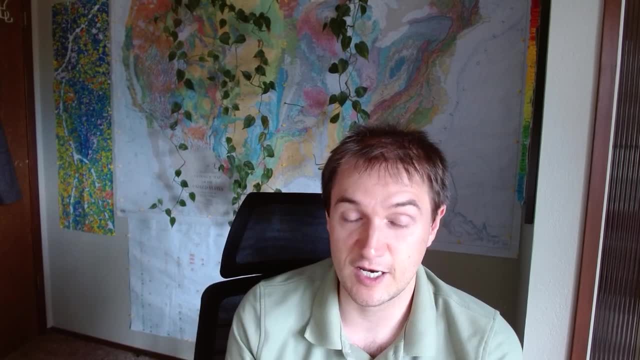 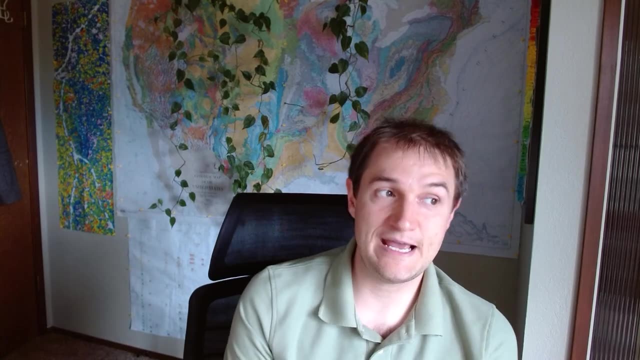 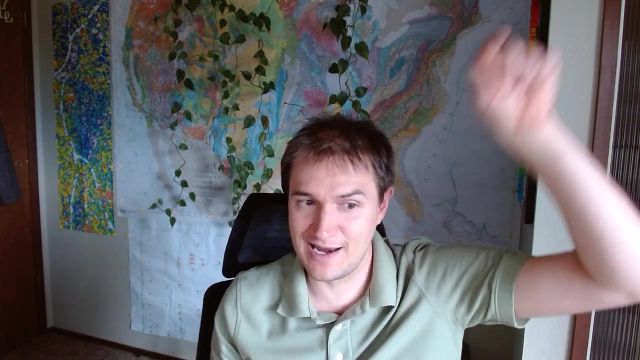 trying to line it up with a remote sensing model. GPS uncertainty is an enormous problem because, as much as we may think that we're good at measuring things with GPS, we're not. GPS is tremendously inaccurate if you go underneath a forest canopy. The reason for that is that the GPS signal comes down from the satellite and it bounces off the 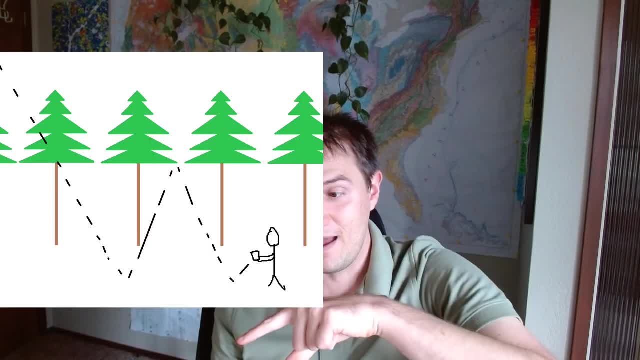 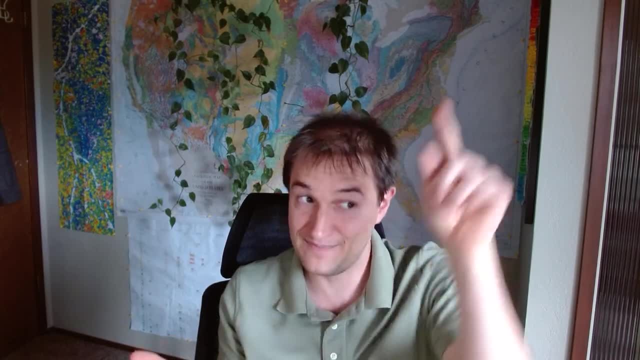 ground and then goes up and bounces off the canopy and comes down and and then maybe it hits your GPS device And in that process you've added something like 30 meters to your location, right, Because it bounces on the ground. Now, to make things worse, GPS accuracy depends on 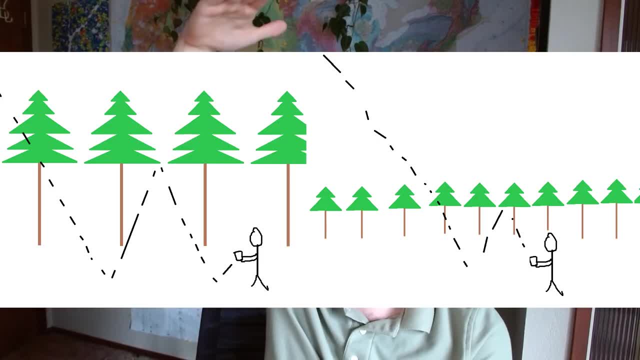 the forest type, right. So if you have a really open canopy with a really dense top that's really dense, you're going to have a really dense canopy with a really dense top that's really, really dense. you're going to have a really dense canopy with a really dense top. that's really. 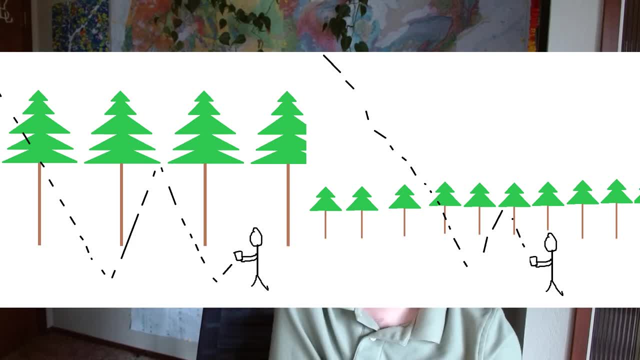 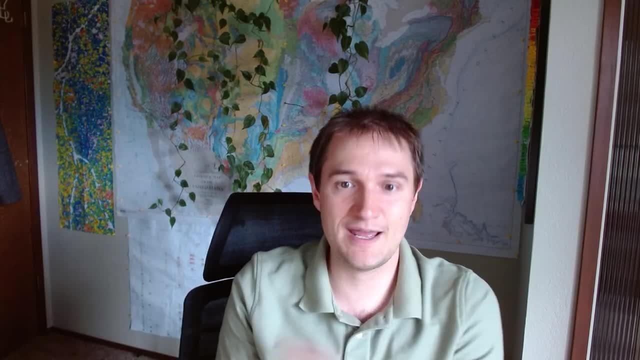 really tall, that's going to be less accurate because there's that much more like area to bounce off of. If you have, if you're in a forest, that basically got like open, clear view to the sky, you're going to get your sub-meter accuracy. Now, the frustrating thing about this is that 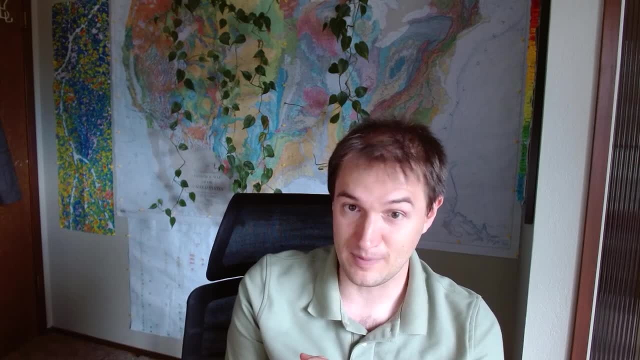 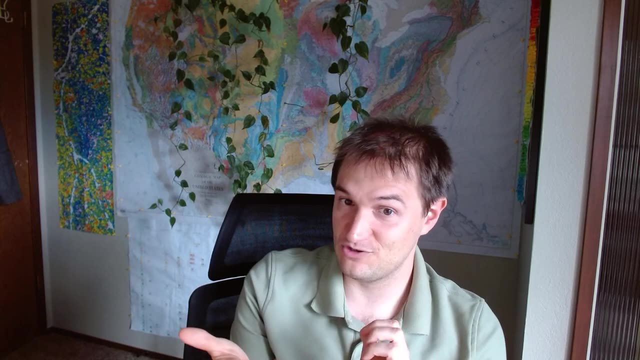 your little GPS device is going to tell you that you're accurate to within a meter because it doesn't know any better, And so that's tremendously annoying, And we have a lot of people going out there in the forest saying that their GPS is actually really accurate, but they're off by like. 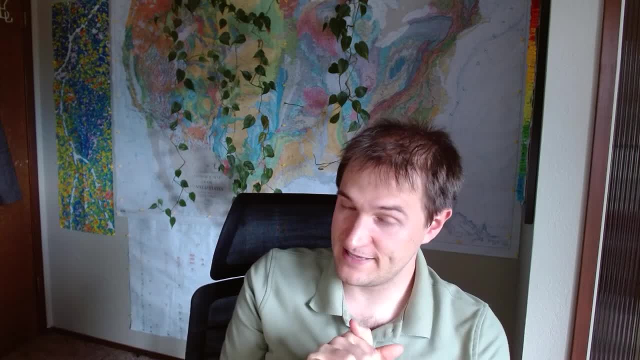 hundreds of meters or something, So. so GPS accuracy is going to be less accurate because they're off by like hundreds of meters or something. So GPS, you know GPSing is really important if you're trying to line it up with remote sensing data. I always tell people that 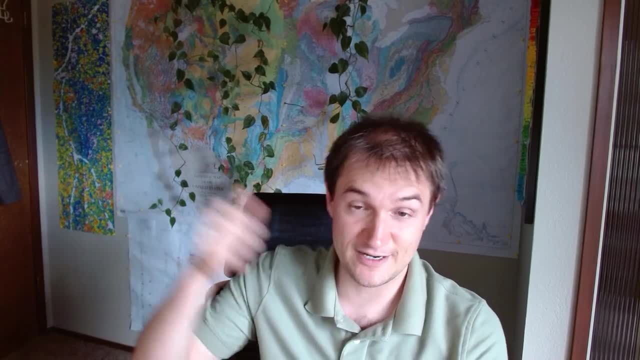 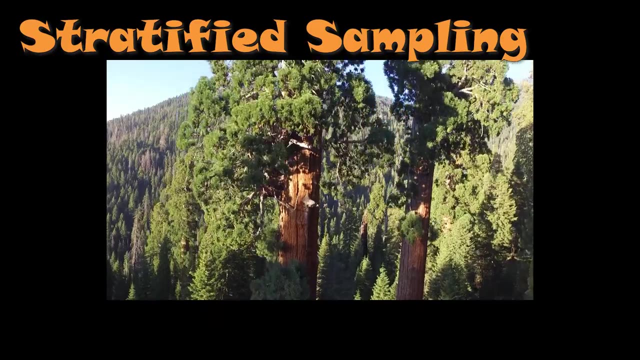 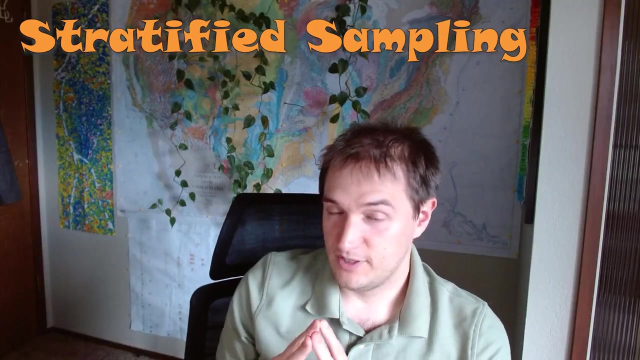 you basically have you take your GPS point but also find some sentinel trees that you can spot from the satellite, so that you can use those to line up your plot. Okay, Now, one thing that we haven't really talked about yet is that you know if there's a lot. 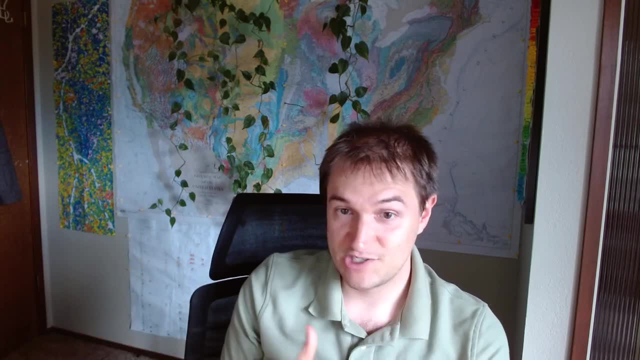 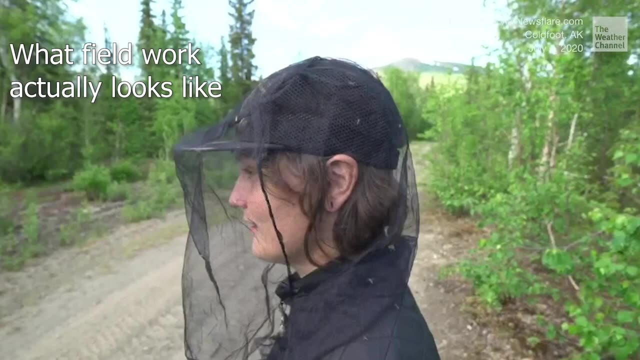 of variability in your forest, you will be stuck out there measuring a lot of plots. This is not good. You do not want to spend a lot of time in the field measuring plots. One of the reasons for this is that it costs a tremendous amount of money to send people in the field and 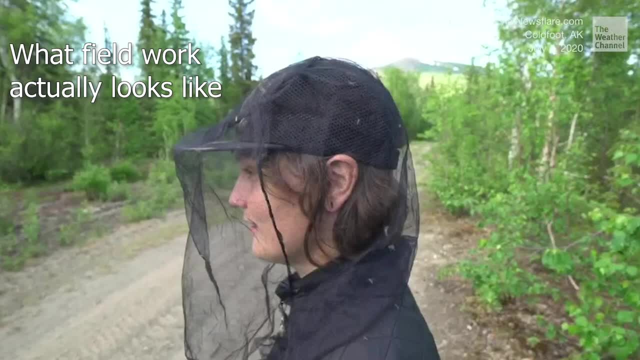 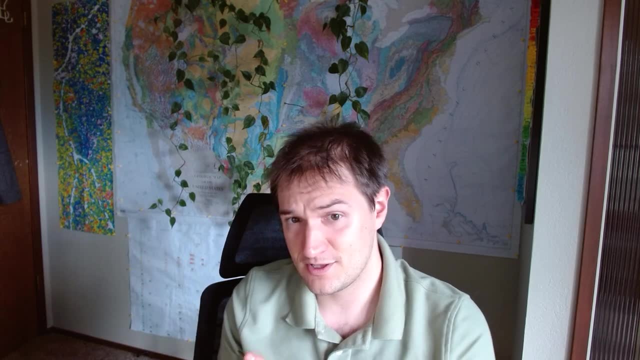 measure trees right. So I mean, I think the US federal government once made an estimate that it costs something like one to $2,000 to measure every plot, but that was a while ago. It probably costs even more than that. So the less time you can spend out in the field, the better. 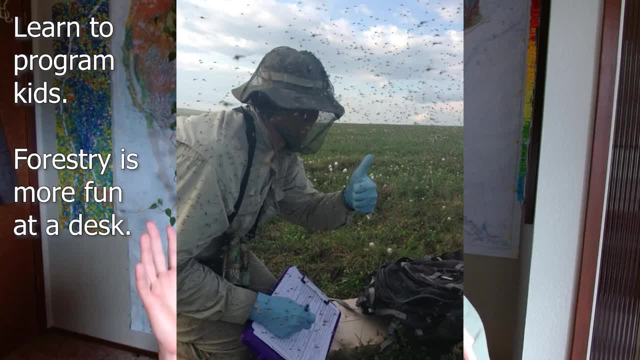 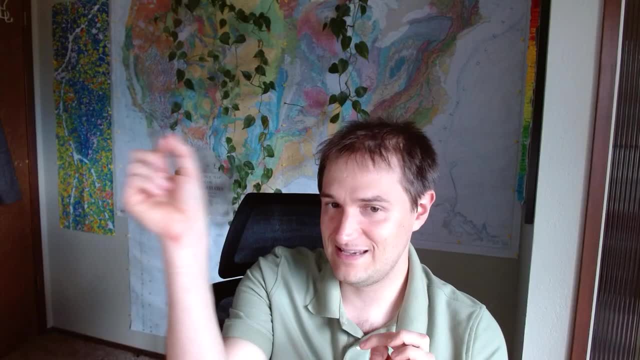 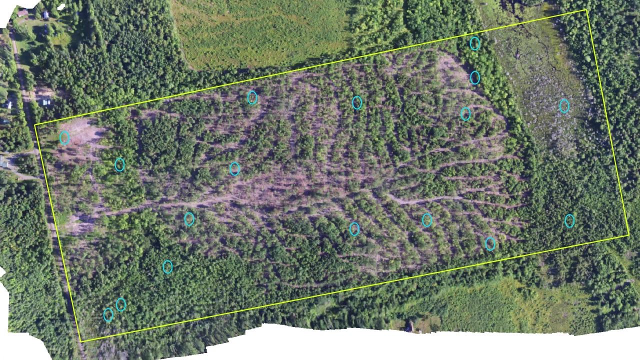 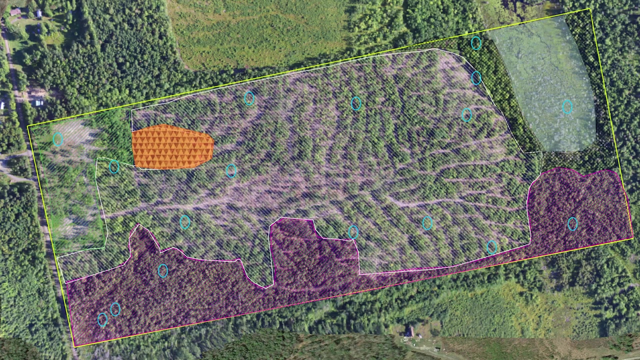 It's also dangerous. I mean, there are mosquitoes out there. So one way that we can reduce variability is to measure trees. So you know, if there's a lot of variability in your forest, you're going to have to take a whole bunch of plot measurements and I don't know 50 plots, or. 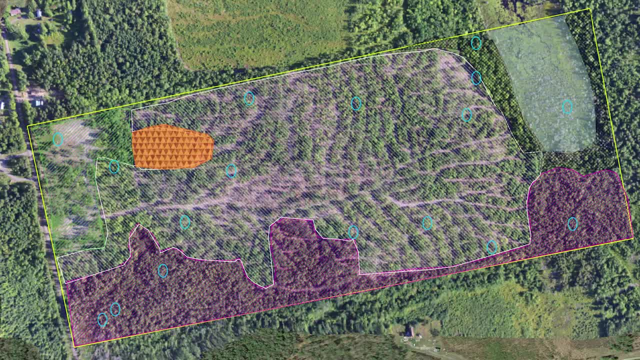 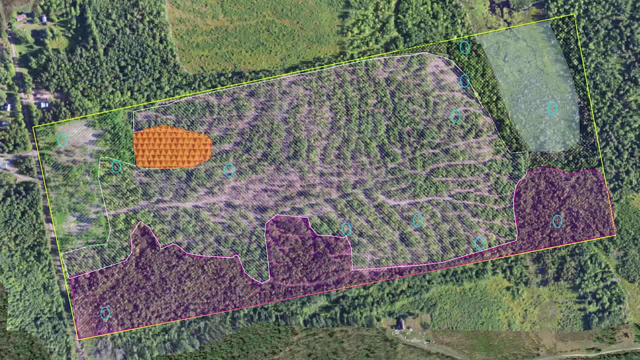 something. But if we measure each strata individually there's less variance because you know the forest is basically the same inside of each strata And so you don't have to measure as many plots if you pre-divide your forest into strata, And that's what a lot of forest 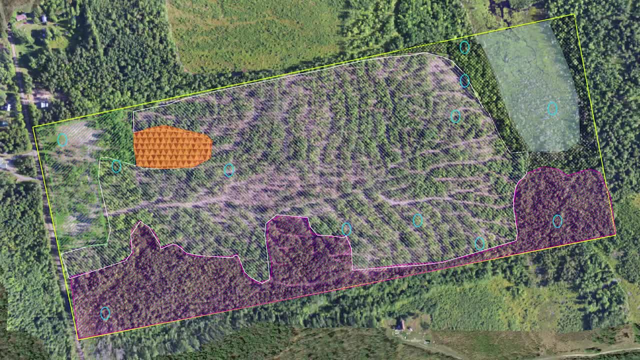 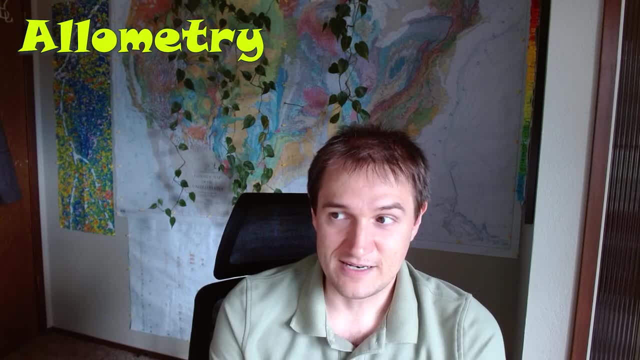 carbon projects will do So. that's perfectly fine. The next thing that I want to talk about is the allometry. Now remember when I said you basically measure the diameter of the tree, the height of the tree and the species and then you plug that into an equation to estimate carbon. 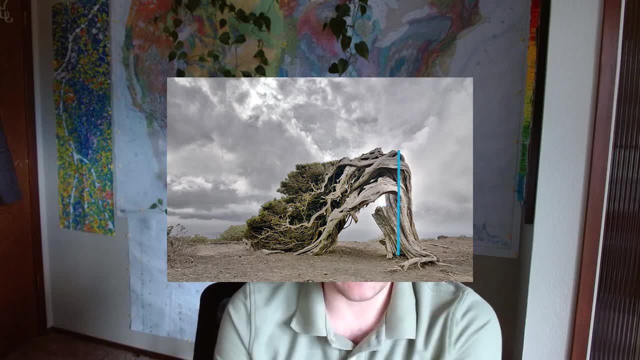 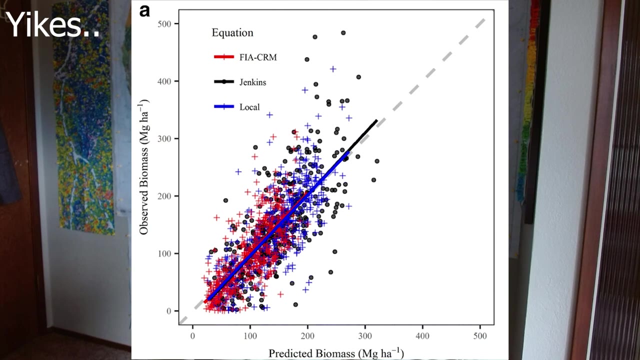 Boy, was that an underestimate of the actual challenges that are faced by doing that? We use these equations to estimate how much biomass there is in the tree, But these equations are often really, really wrong. So, first of all, in the developed world, 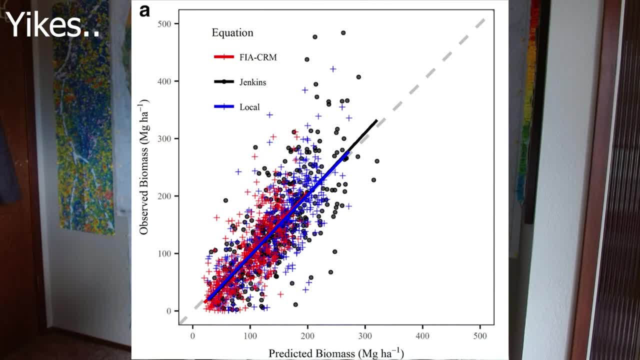 we spend a lot of time working on our equations. We've spent, we've poured millions of dollars into making sure that our equations are correct, And so in the developed world we have very good equations, And one thing that's nice about the equations in the developed world is that 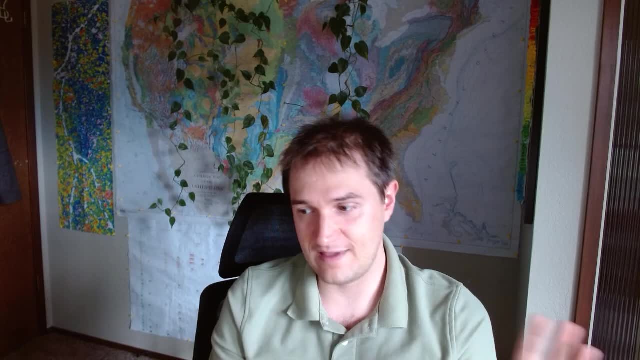 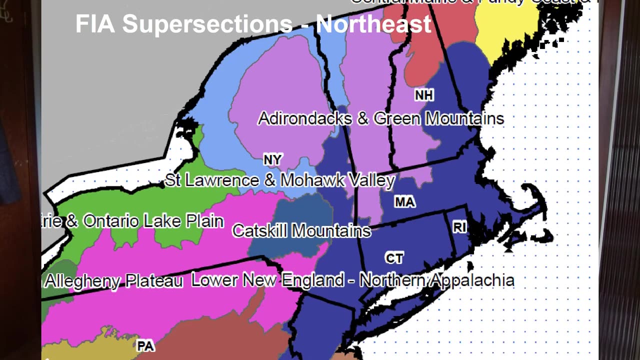 we separate them into areas, right. So in the US there's these areas called supersections, where they're basically like ecosystems, And there's a separate set of equations for you know, the ecosystem in Michigan than there is for the ecosystem in Wisconsin, maybe. 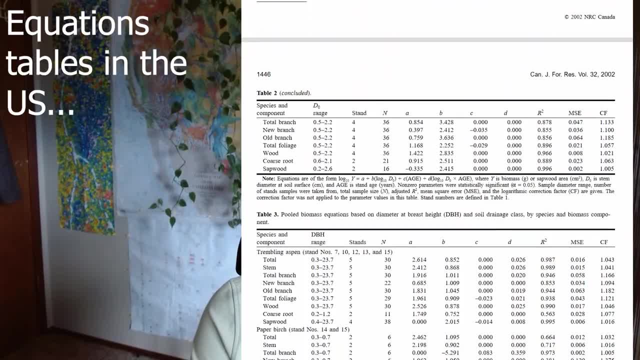 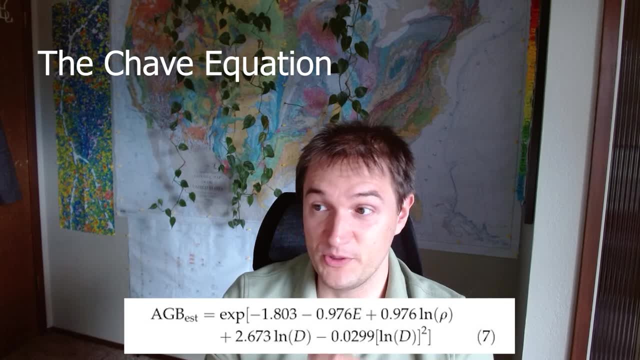 Outside the developed world it's the wild west, And a lot of the time people are just using a single equation for every single tree. In a lot of the tropics we just use one equation. It's called the Chauvet equation, And well, I mean it is what it is. 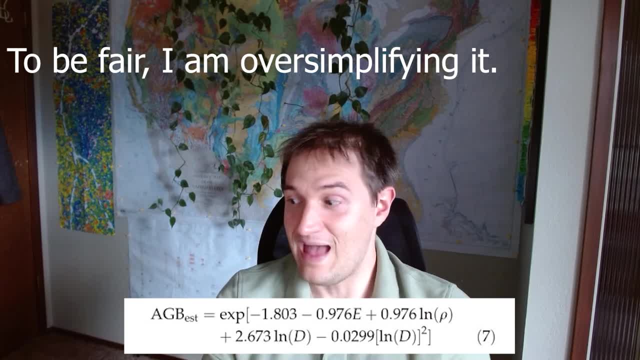 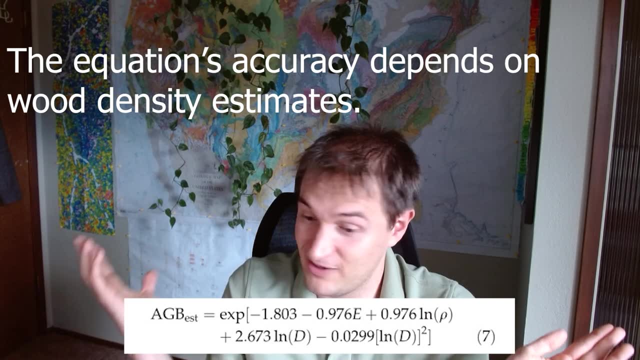 The fact is there are thousands of different tree species in the tropics and nobody has done the work to really quantify the, you know the biomass for this species or that species. So we all kind of just converge on one. Let's talk about where some of these equations go wrong, First of all. the only way you can actually develop these equations is by cutting trees down and measuring them on scales. People don't want to do that. People especially don't want to do that if they're massive trees. Nobody wants to cut down a tree and then dice it up into a thousand. 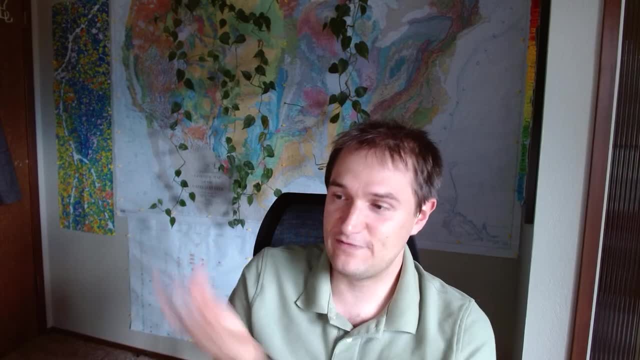 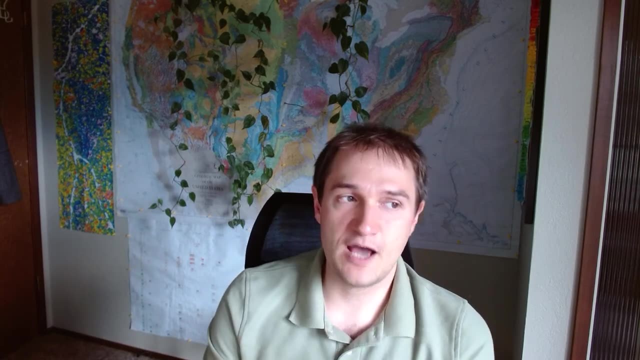 little pieces if it's a thousand year old old growth. Nor do they want to do that if it's a thousand year old old growth, and you could have been selling that for two by fours, right. So the equations you know, oftentimes equations for entire countries, may be based on something. 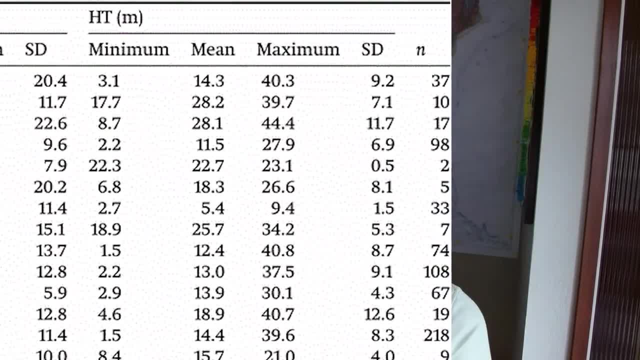 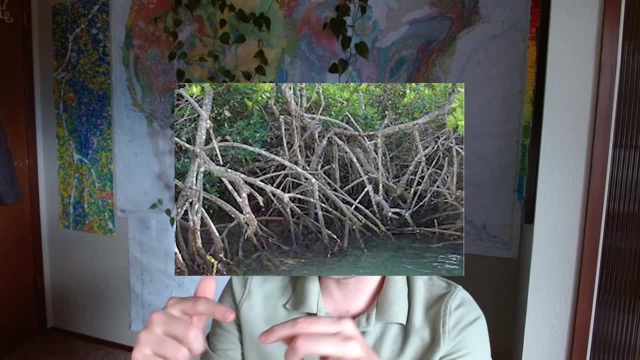 like 50 trees, 50 trees that have been cut down. Now anyone who's actually looked at a tree is capable of saying that just measuring the diameter of the tree at breast height and measuring the height of the tree is not enough information to really 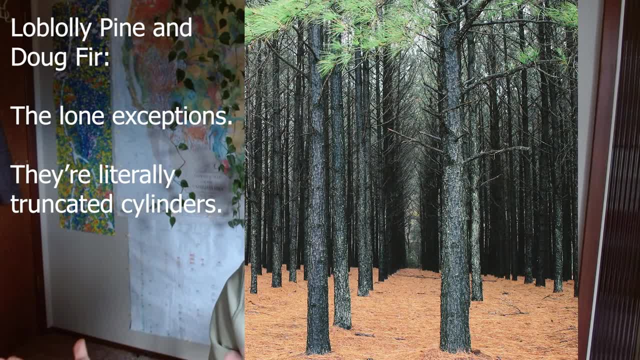 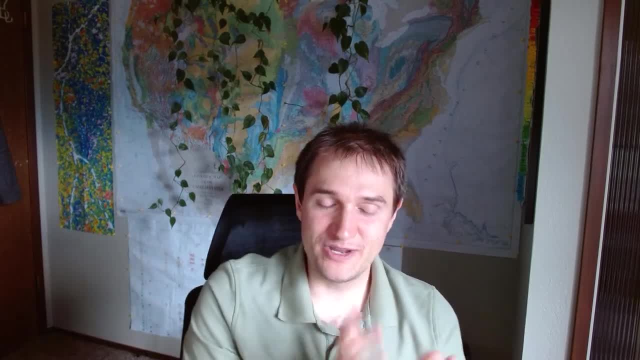 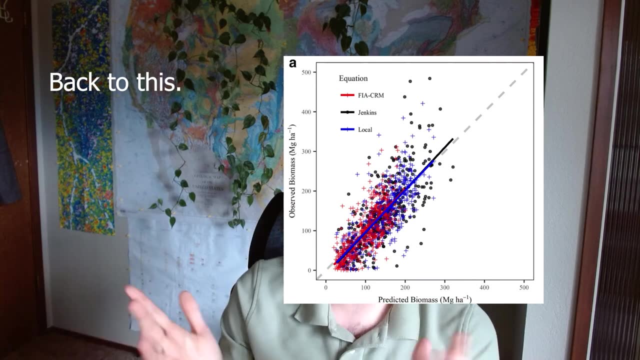 figure out what is going on inside that tree. So we are massively oversimplifying these trees with these equations. One thing that's really challenging about these equations is that the error around any given prediction is enormous- 30,, 40,, 50 percent. So it would be nice if we 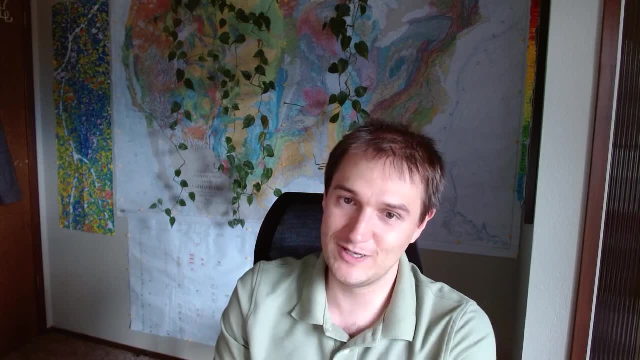 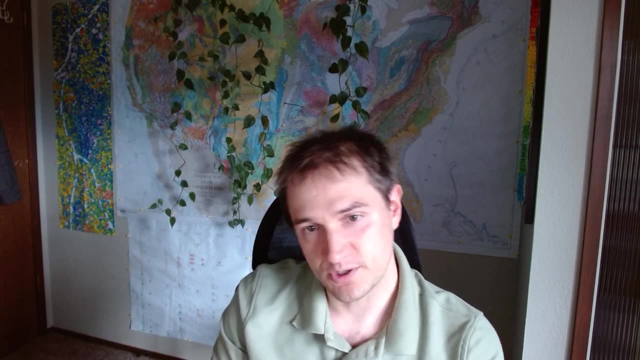 could say we could go out in the field and measure a tree and know how much carbon there is, but we really can't. We, you know, we do our best. One thing that people will often tell you is: okay, this is a tree, This is a tree, This is a tree, Let's measure it out. Well, if you have a tree, 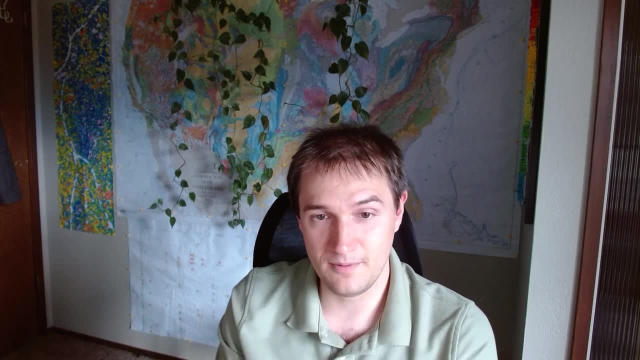 then you can measure it out. You can measure it out to come out of 10,000 and it doesn't level out for 10,000 percent for a particular tree. But if you're measuring 10,000 of them, then the errors. 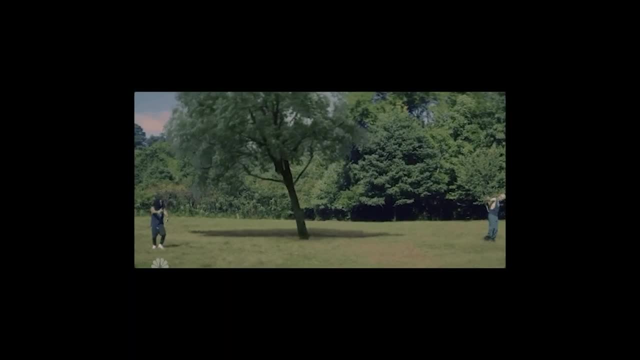 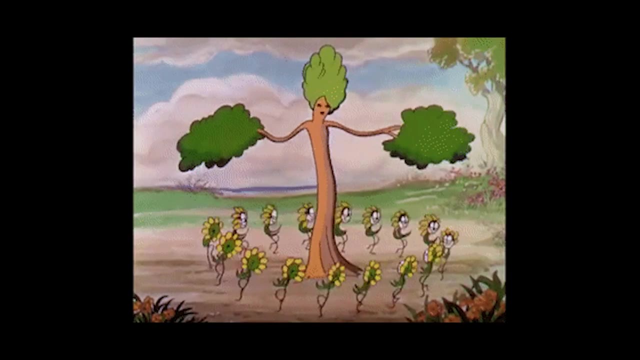 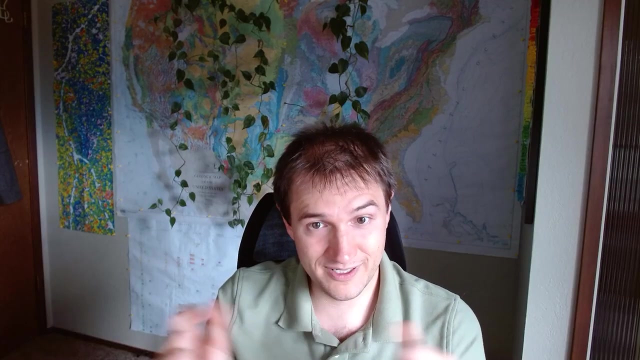 will level out and you'll end up getting a very good, like very good, number on how much carbon there is in 10,000 trees. Don't sweat it, It'll all come out. I'll come out in a wash. It'll all come out. I'll come out in a wash. 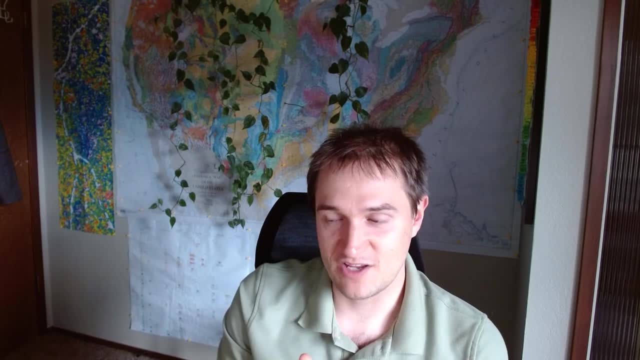 No, No. The reason for this is that the errors are such that they are so gonna be so much better than what they were made to taste. error in allometric equations is very, very spatial in nature, and what i mean by that is that, if you 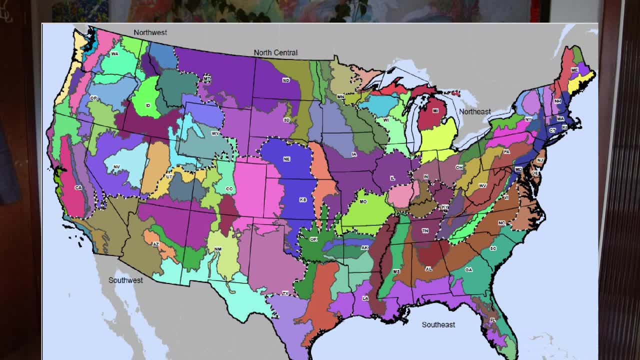 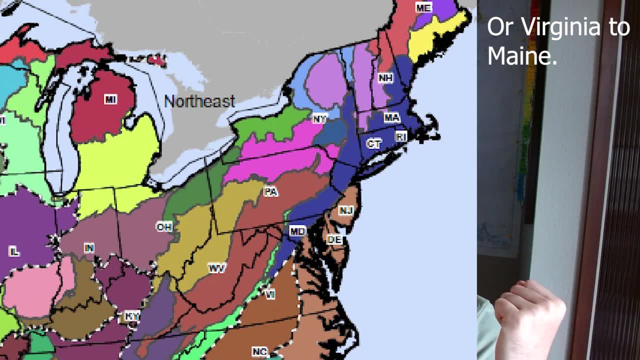 do have your super section. uh, you may have an equation that corresponds to all the trees you know from connecticut to the top of maine, and that's all great, but the fact is, red maple at the top of maine grows very different than red maple down in connecticut, and, and so it's just. 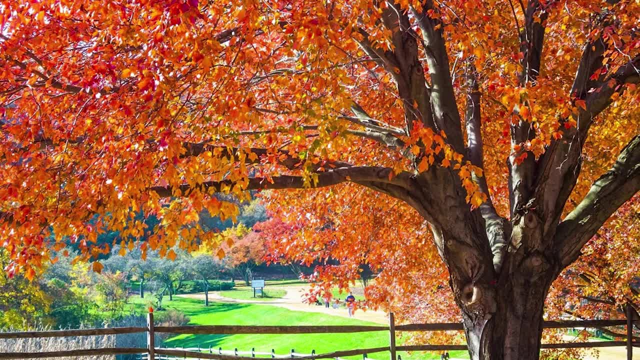 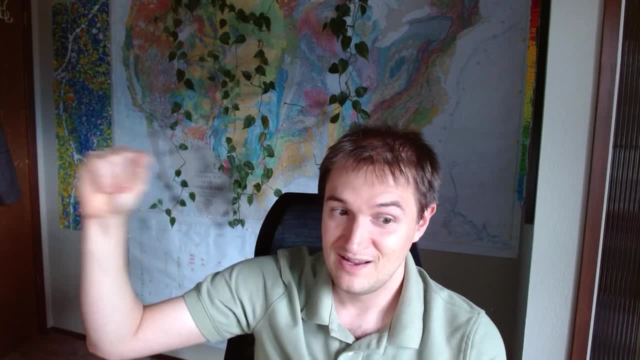 not appropriate to apply that equation, and so your allometric equation may be doing really good across all of the trees in that area. but you know, if you're focused in on a very specific section, it's going to be off, and if it's up at the top of maine it's going to be over predicting by 20. 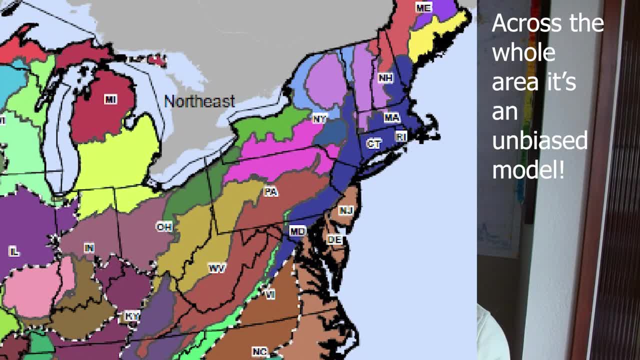 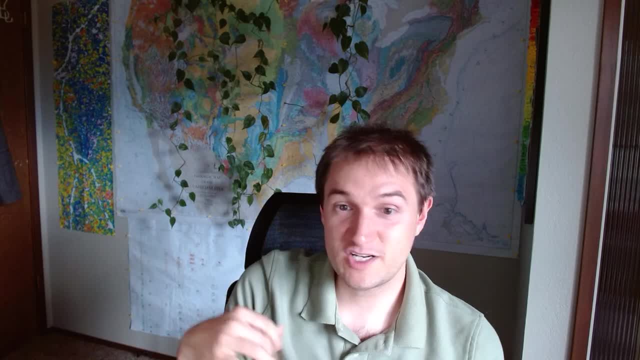 and if it's at the bottom of connecticut, it's going to be under predicting by 20, because the trees are smaller up there and bigger down there. this is only one small problem. it gets much more complicated than that because even within a microsite- uh, the allometry is wrong. 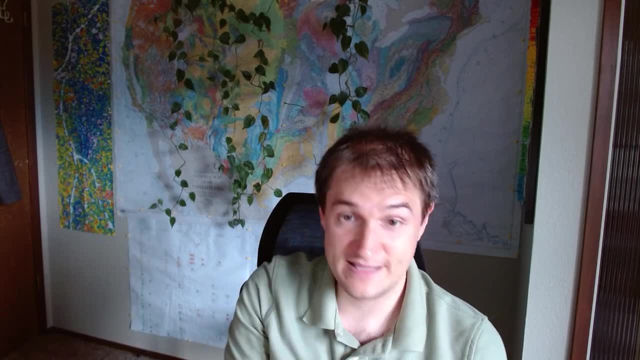 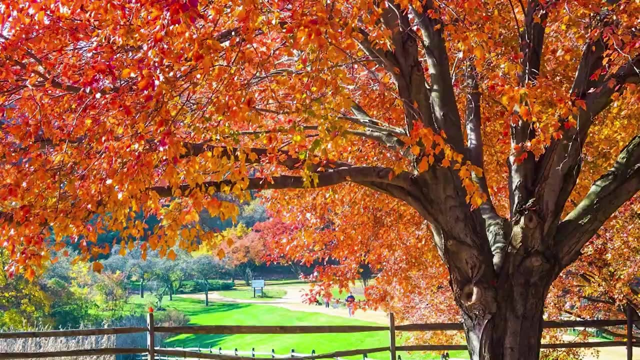 in different ways. so imagine, you know, at the base of a mountain, measuring a red maple, it's a much more productive site that you're going to basically underestimate how much carbon there is with your allometric equation. and then imagine going to the top of that mountain, on the north side of the mountain, where it gets even less light. 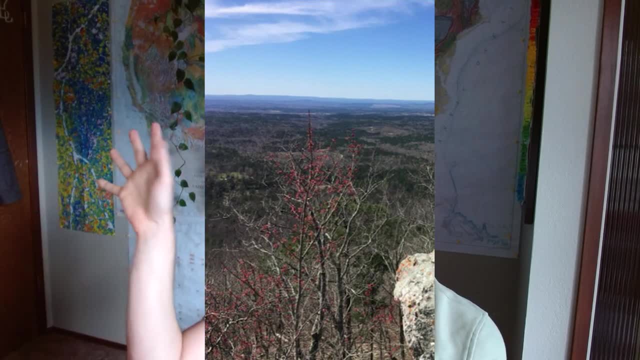 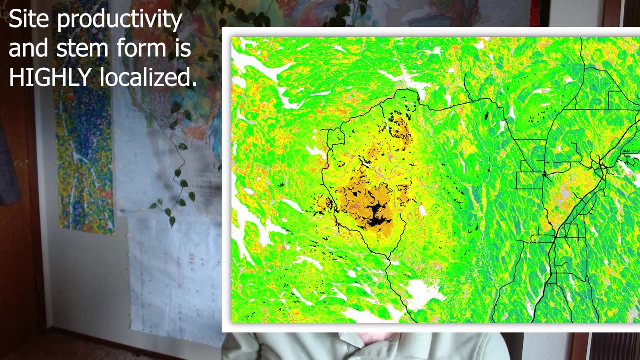 uh, the red maple is going to be all gnarly and twisted and it's going to grow funny and you're going to be overestimating carbon by 20. this is the problem that we face with allometry. and guess what? uh, we brush this under the rug, we don't deal with it at all. every single carbon. 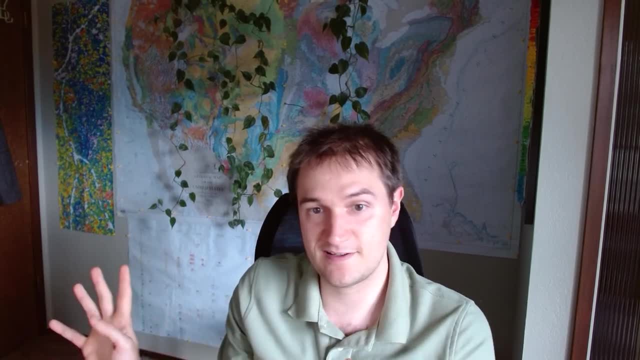 project is going to be under the rug. we don't deal with it at all. we don't deal with it at all. every single carbon project is going to be under the rug. we don't deal with it at all. every single carbon out there ignores this error. we just we pretend it doesn't exist. and i think you know to some. 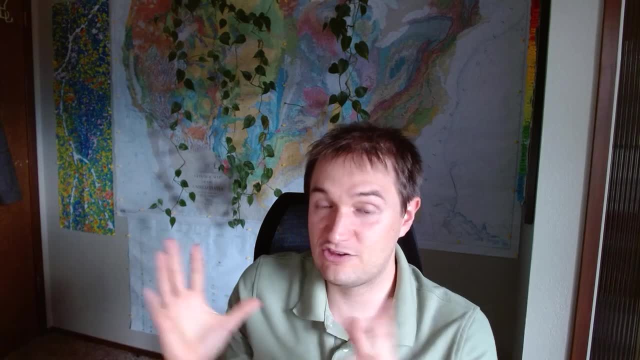 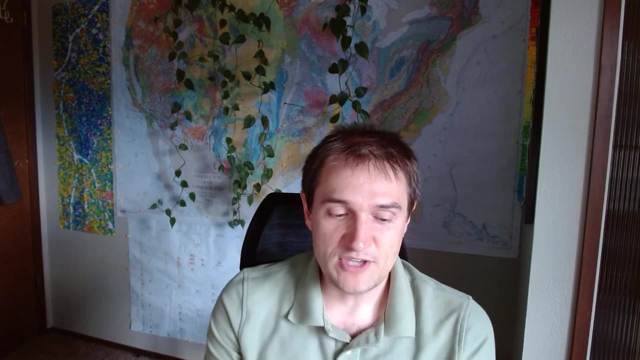 extent we have to kind of do that, we have to throw our hands up in the air, but to another extent we're just pretending that like a massive amount of uncertainty, like 20 to 30 percent, just doesn't exist at all. so that's allometry and i'm going to revisit this topic in another video. 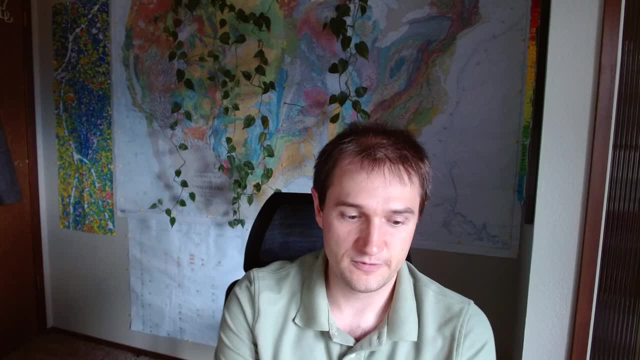 because it really does deserve an entire video to itself. uh, so we've talked about how we can measure trees within plots. what we're going to do is we're going to measure trees within plots and we're going to measure trees within plots, and we're going to measure trees within plots and we're going. 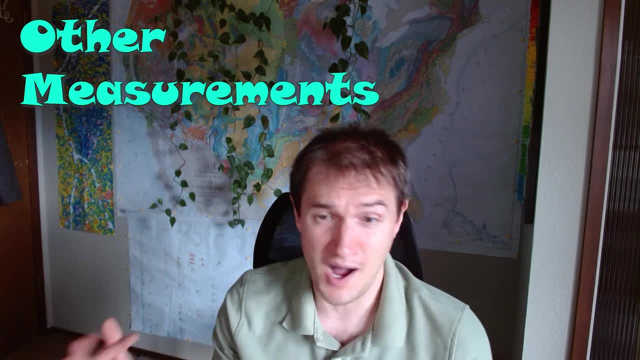 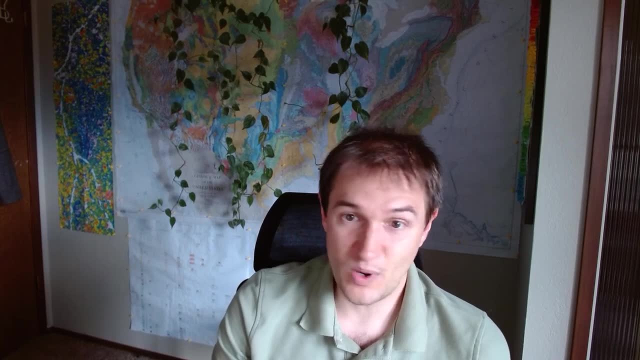 what other good information do we often need to measure on plots for for forest carbon projects? well, growth and yield is another good example. it's one thing just to measure how much carbon there is on the plot today, but what we really want to do is predict how much those trees are going to grow. 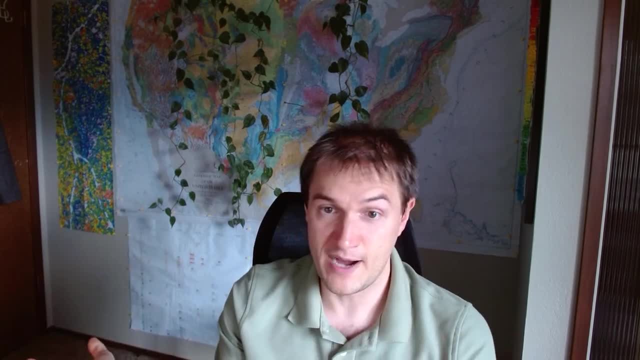 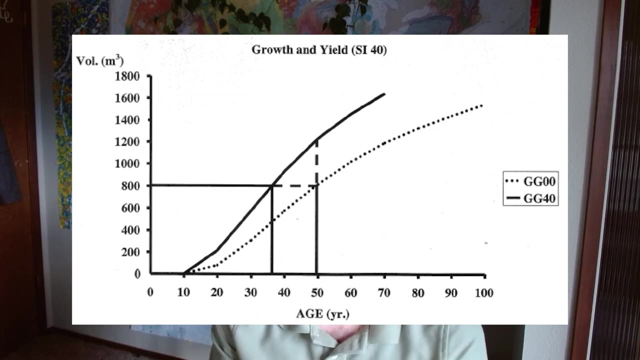 in 5, 10, 15 years. this is a whole nother set of modeling and, like i've often said, trees grow along an s-curve. uh, the growth rate depends on the site quality and on the soil type. uh, and you know, the growth rate depends on the site quality and on the soil type. uh, and you know, basically, you know. 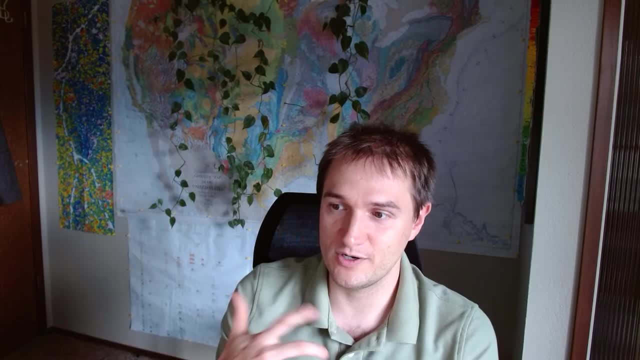 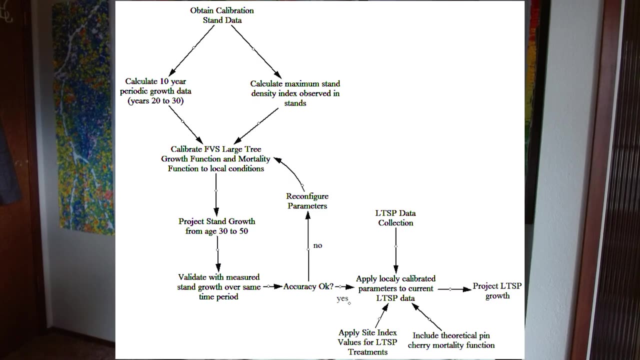 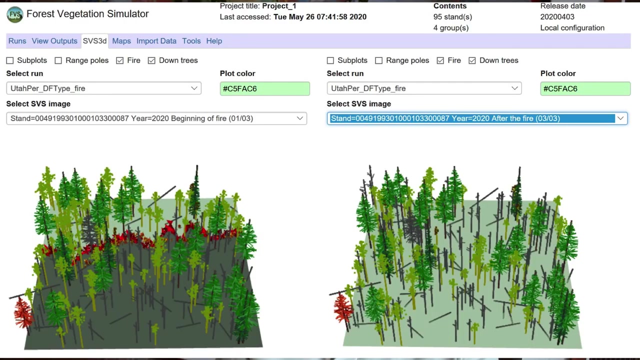 basically any time that you're doing like tree planting or or forecasting economic returns from carbon projects, you should be doing very sophisticated growth and yield modeling. now in the united states we've got some very nice public tools for doing that. the forest vegetation simulator is one that everybody uses and it's very accurate. it can tell you very, very reasonably if 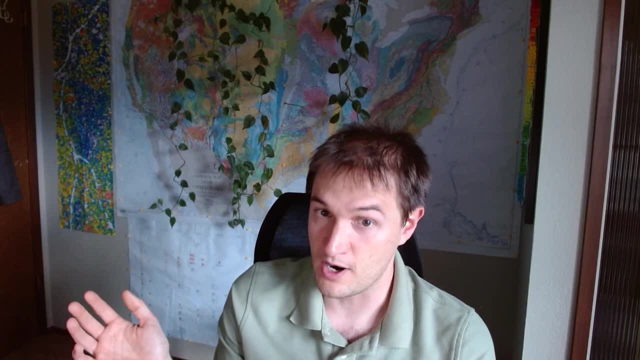 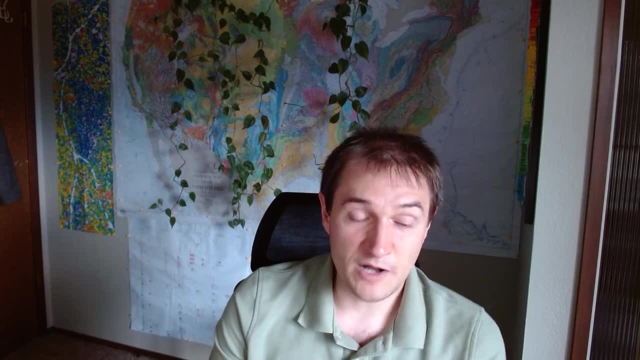 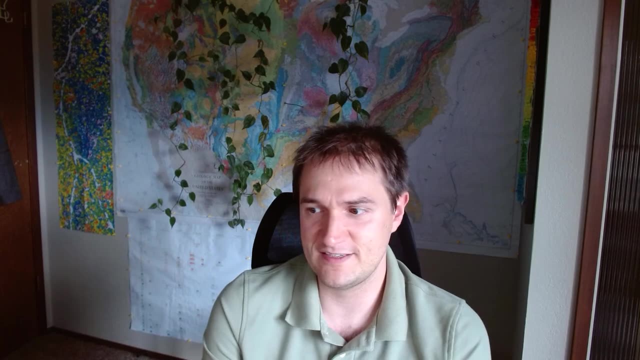 and this is the soil type, and this is the soil type and this is the the site index and all that um, outside the united states it's just the wild west. we have no idea how fast tropical trees grow, and so a lot of these like reforestation projects that are taking place in like 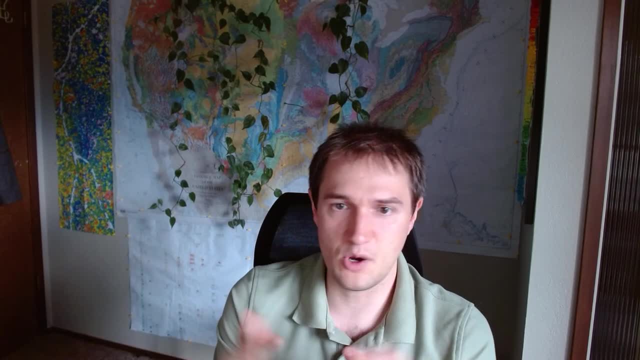 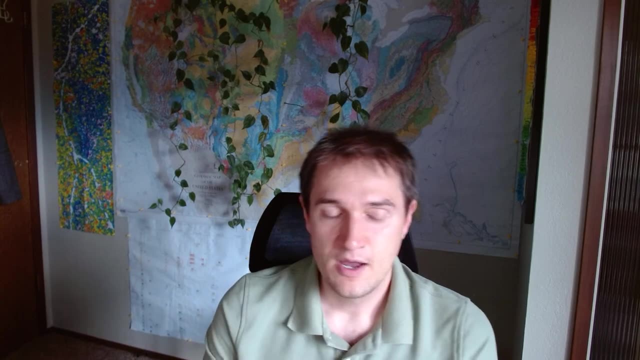 peru, where they're planting native rainforest. we have no idea what the returns on those carbon credits are going to be, because the models just don't exist. there's nobody out there like actually doing the science. uh, if you're talking about commercial species, uh, there, there's much better. 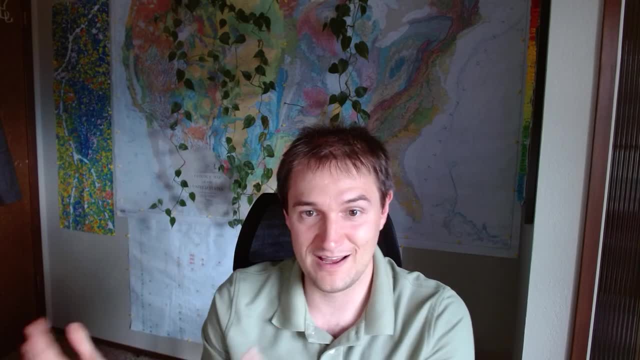 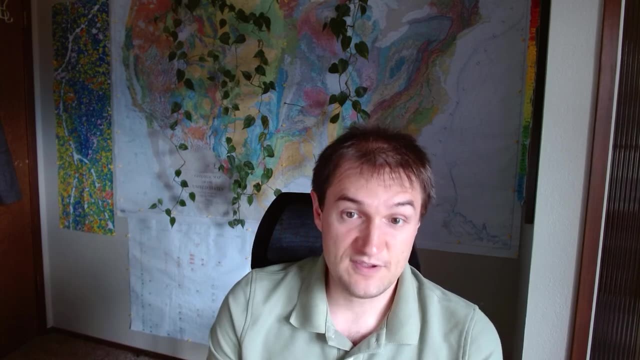 data. there's always people like categorizing the growth rates of pine or eucalyptus. you're talking about wild, native, tropical rainforest species. we, we just don't know. uh, the other things that you can measure, uh, you can measure wood density. so wood density is basically tied back to 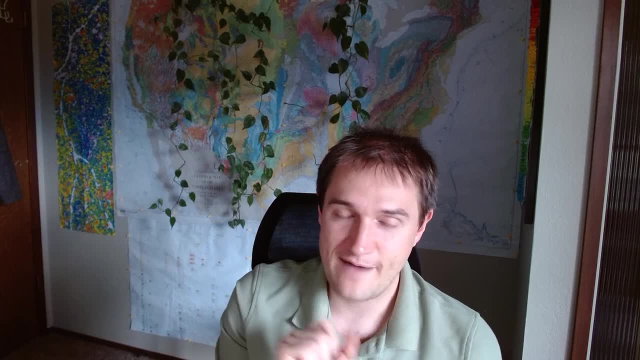 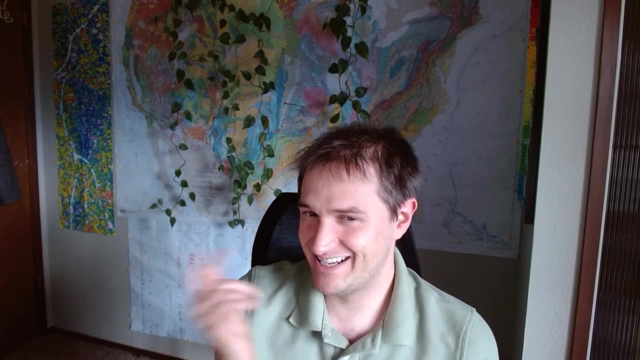 the quality of your allometric prediction. uh, and if you, if you have a better estimate of wood density, you can get a better estimate of how much carbon there is in the forest. now, does it really matter how much carbon there is in the forest? like i said, we brushed that. 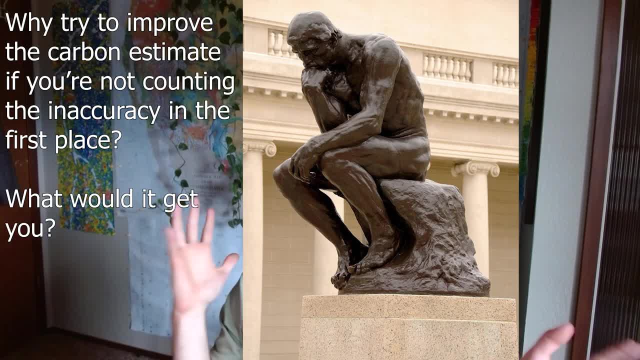 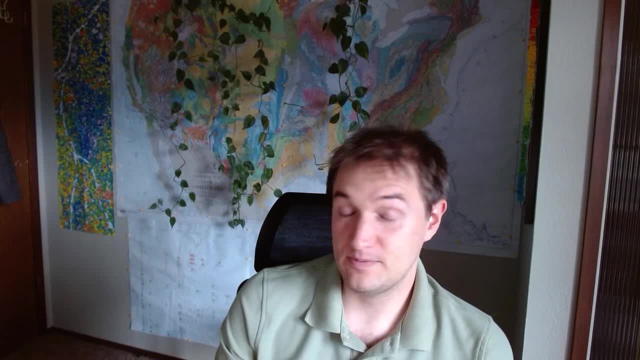 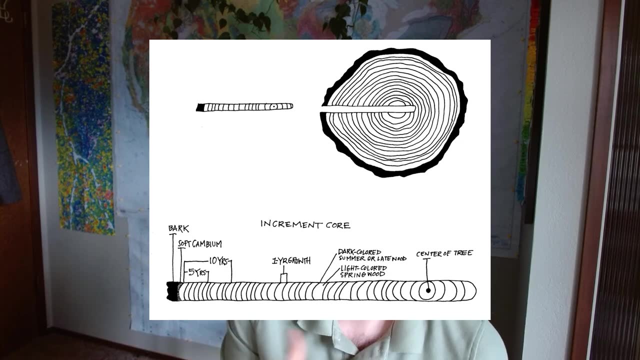 whole allometric uncertainty right under the rug. so who even cares if we're wrong on that? so i'm. most people don't measure wood density. um, you can measure productivity. so, for example, by measuring the, the growth rate, the tree rings, uh, and the age of the forest, you can basically measure how fast. 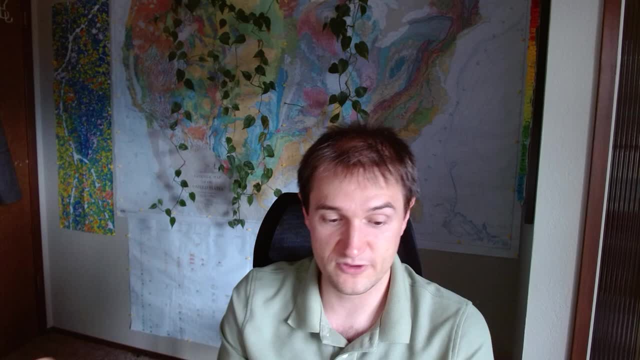 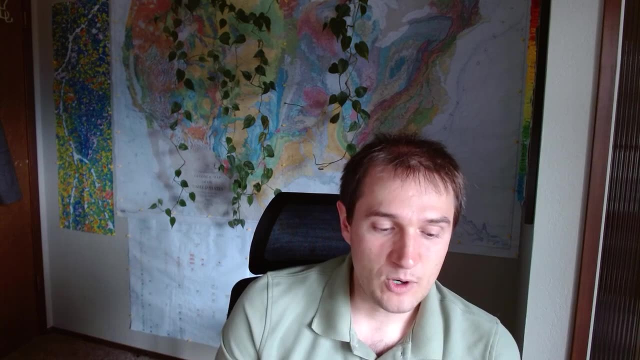 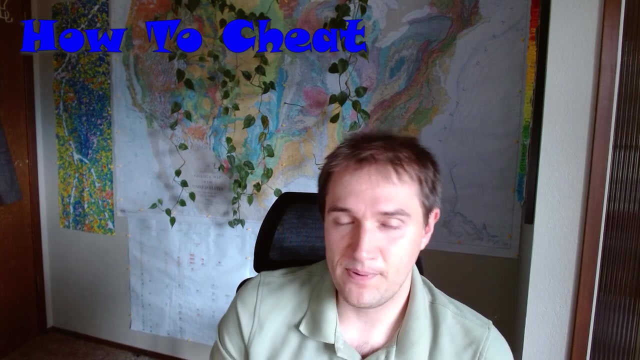 the trees grow, and this is very important for developing growth and yield models, uh, you know, for predicting how you know what you're gonna, what your returns are gonna be in 30 years. um, okay, so we've talked all about some of the nitty-gritty details. let's talk about how carbon projects. 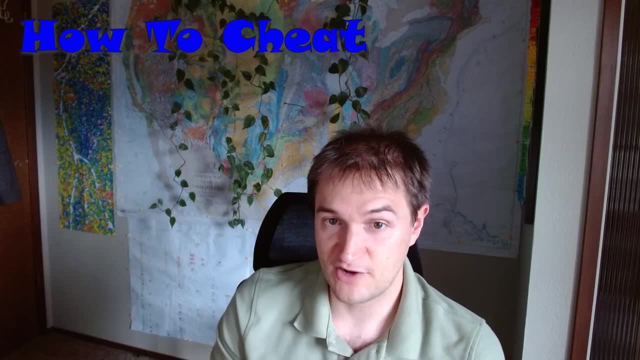 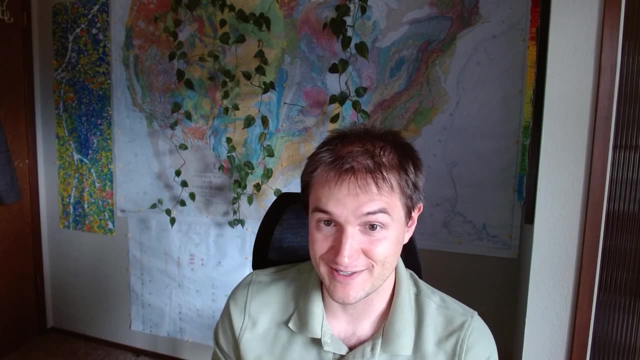 are used in the system. one way that they game the system is that some vera projects don't have any specifications around which allometry you use some vera projects. let you use your own allometric equations. guess what? there's a whole bunch of carbon projects out there that have used their 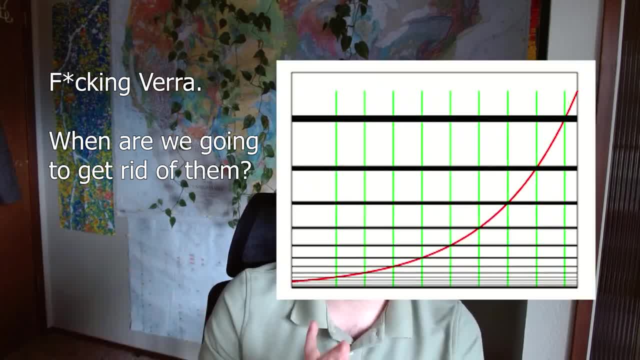 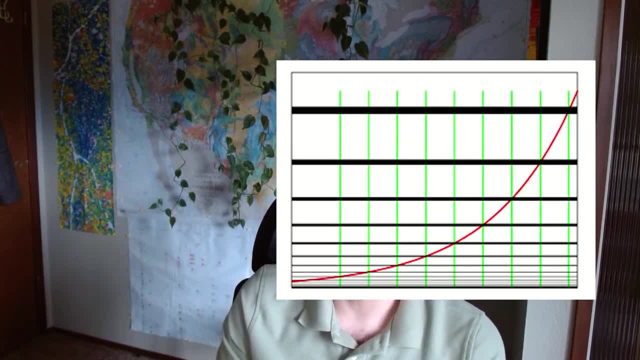 own allometric equations that are, and surprise, surprise, they end up estimating that there's far more carbon than they should have. uh, there was a project in mexico, for example, where they were like planting eucalyptus trees and like over predicting their carbon stock by like 25. 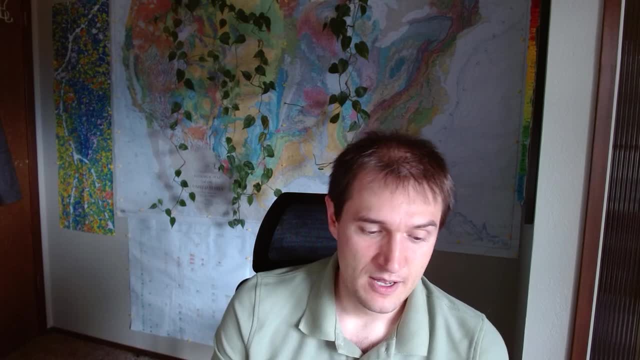 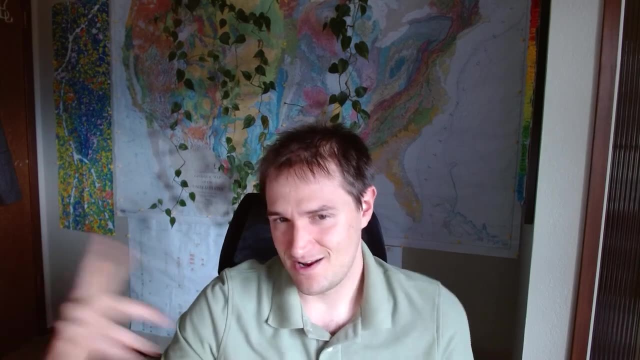 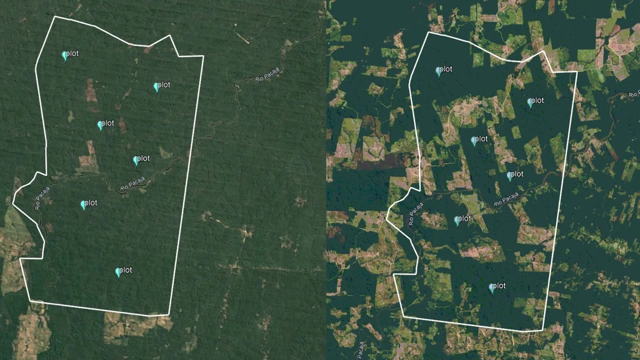 um, so you could use bad allometry. that's a problem? uh, you could know where your plots are. so picture this: you're a project developer with sinister intent, uh, and, and you? you lay out your plot system to measure your trees, and you know exactly where you've put all those plots. now let's. 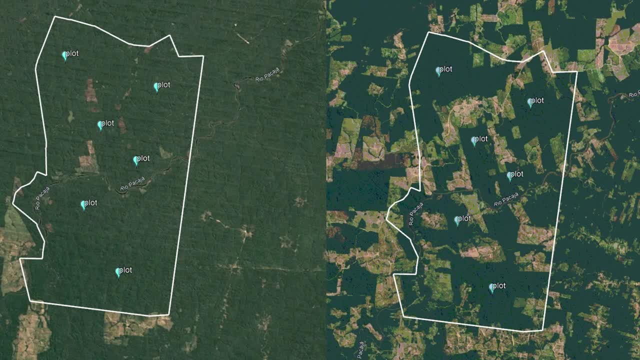 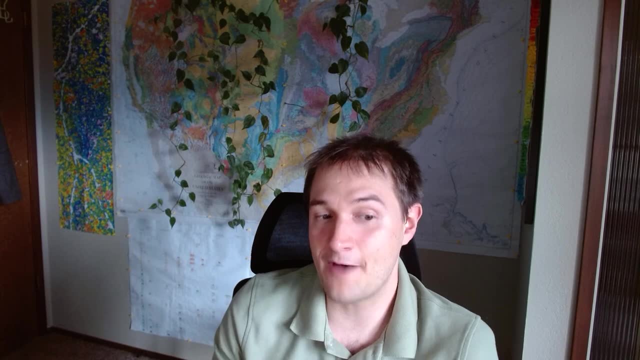 say, you want to cut a bunch of trees down without anyone detecting it. well, you can basically just go and cut around the plots, and this has happened, i think, a couple of times. what the problem is is verifiers who are measuring the trees will sometimes share the locations of the plots. 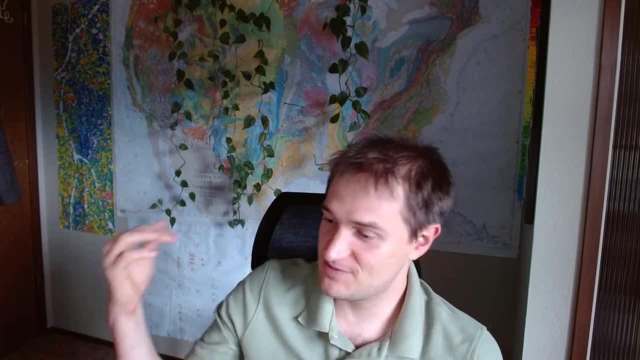 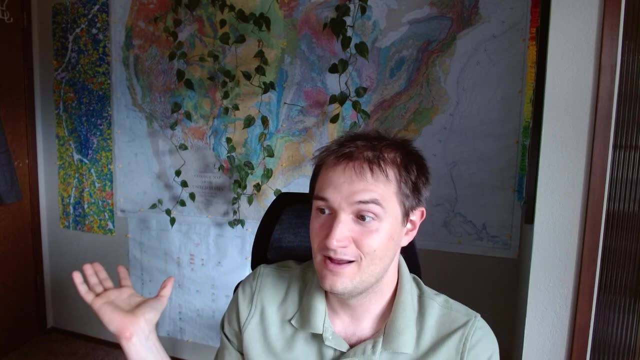 with the people who want to cut the trees down, and then they just basically cut around the plots. you go and re-measure the plots after 10 years. oh, what do you know? the forest is growing, but in reality, a bunch of the forest has been clear-cut. another thing that can go wrong is you can just 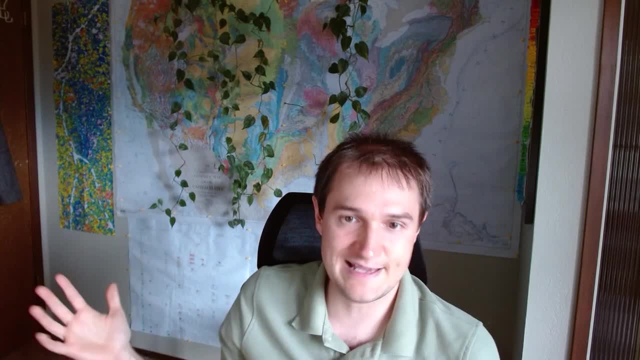 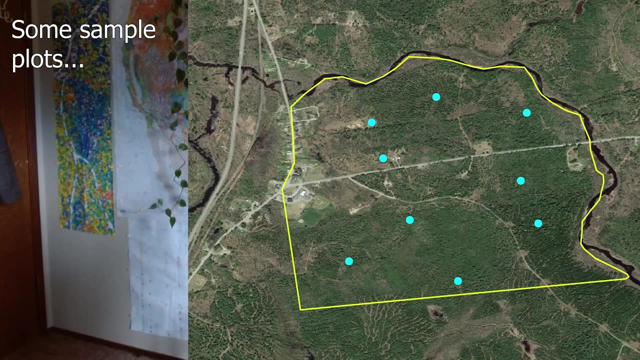 miss things. so you're going out. you're throwing like 50 plots out there on the landscape. what are the odds that you're going to capture the really weird situations? a lot of the time, especially the largest trees store a disproportionate amount of the carbon and so you know you could have really 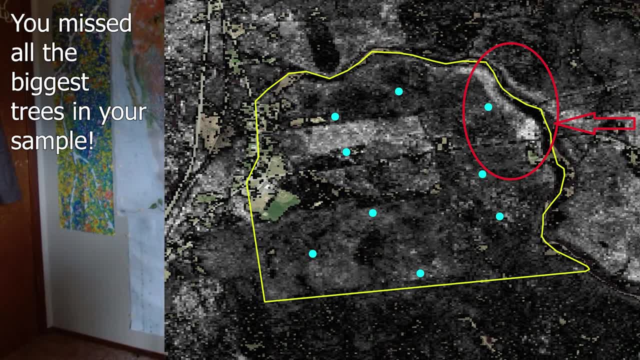 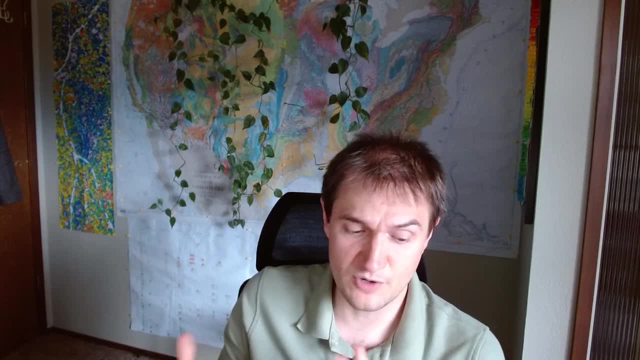 big trees, like sitting out there, that are just, you know, not being captured by the plots. they just happen to not, and so this is one of the nice things about remote sensing is that you're measuring everything and there's no way to hide the fact that you. 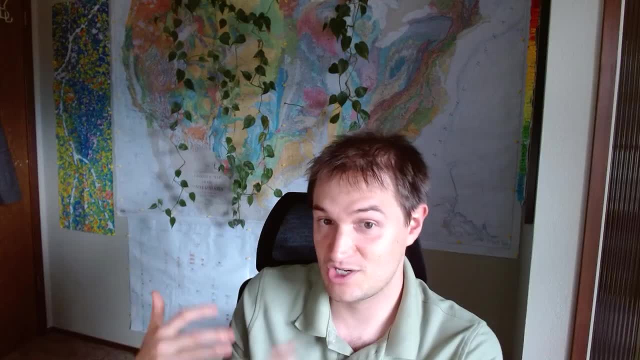 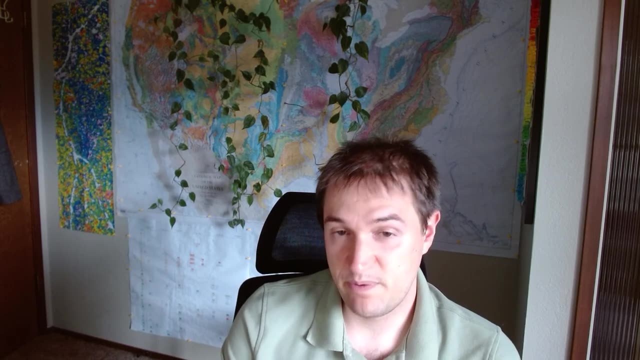 cut down your biggest trees or that you're missing some of your biggest trees and you really should get more credits, whatever. uh, another thing that i want to talk about is that there are forestry projects out there that don't require you to measure the trees at all. 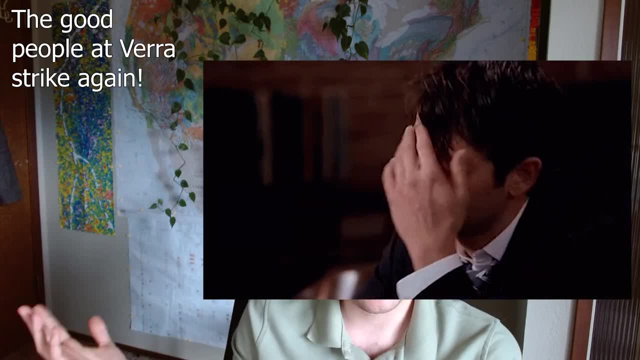 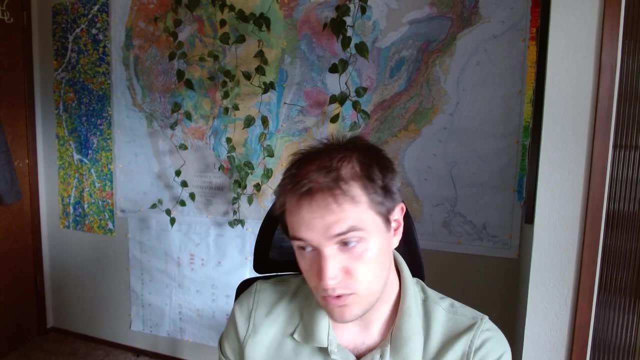 I often say that VERA is a buffet table of crap. You can pick and choose exactly what you want to do with a VERA project and you can get away with anything. Well, under VERA protocols, you're allowed to not measure a single tree in your forest. Now you're not using remote sensing. 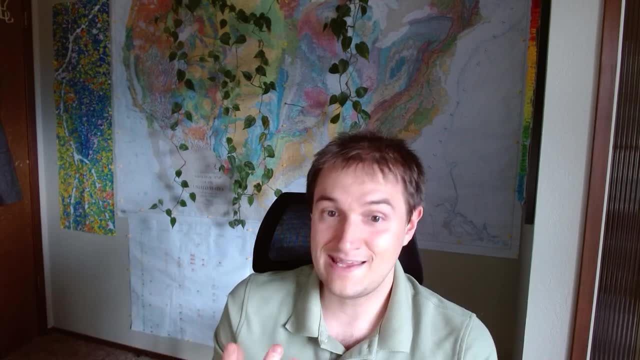 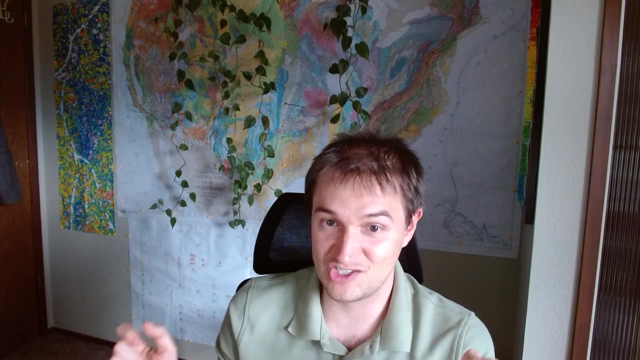 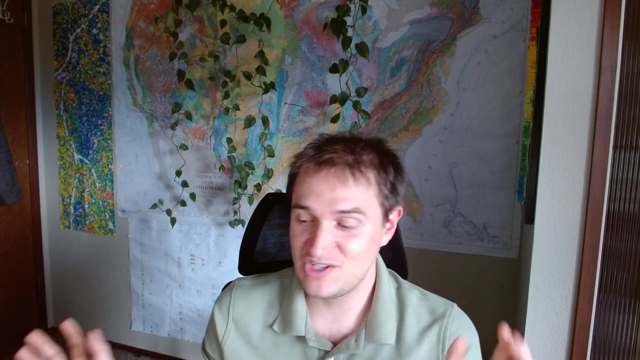 You're not measuring trees by hand. The way that they come up with their estimate is by taking a regional average, And so some VERA-avoided deforestation projects literally just allow you to take the average for the entire state- an area like bigger than most countries sometimes- and just say this is the average carbon in our project. 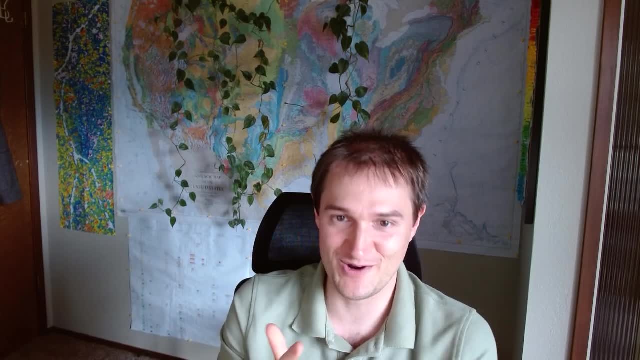 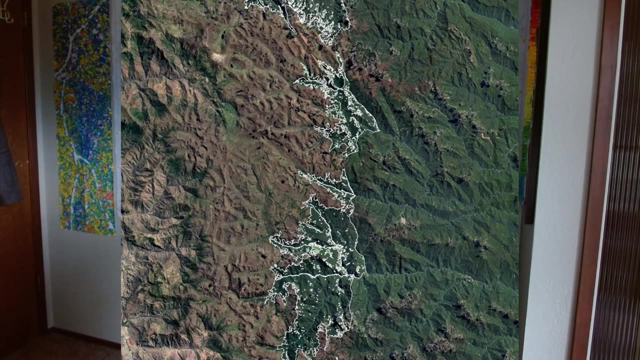 Now anyone with the slightest bit of forestry chops will tell you that is a really dumb idea. There have been numerous VERA projects that do this and, surprise, surprise, you know they're taking place on top of like, in like, high alpine mountains. using the state-level average, 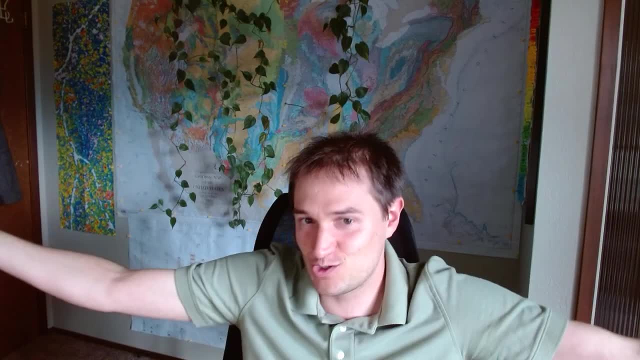 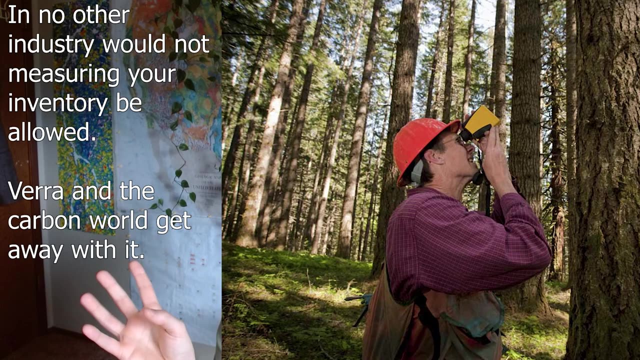 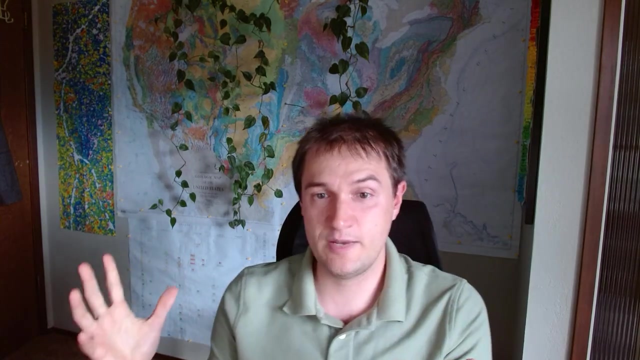 that you know has far more biomass than their actual project area. Anyone in forestry will be able to tell you that one forest does not equal another forest. The amount of carbon stored on the landscape is very different from one plot to another, In fact. here's an example. 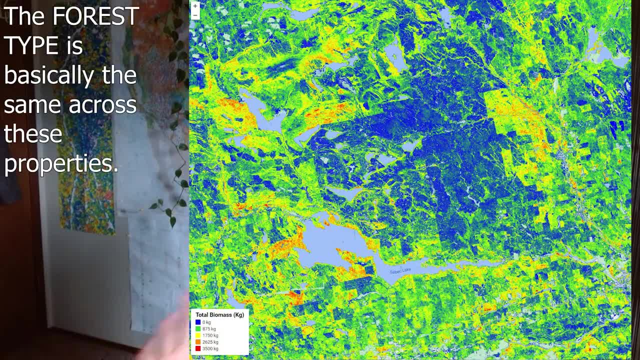 Here's an example of a carbon map that I made a while back. It's very accurate. It's using remote sensing. Imagine drawing a property in one of these low density areas and then using the average for the entire state. Really bad idea. 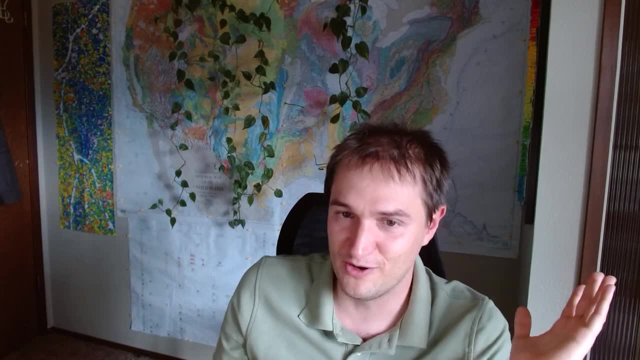 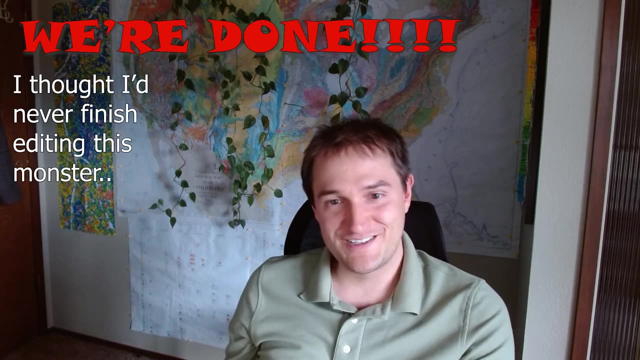 So you know there are projects that do this just to immediately score a zero for Renoster's criteria. But you know they're out there. So that's a thorough sampling of forest sampling. We've talked about plot measurements, uncertainty. 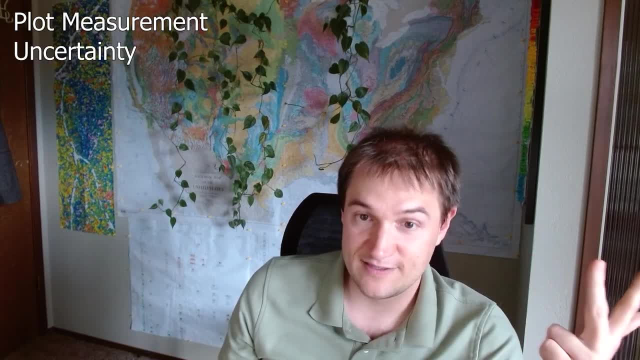 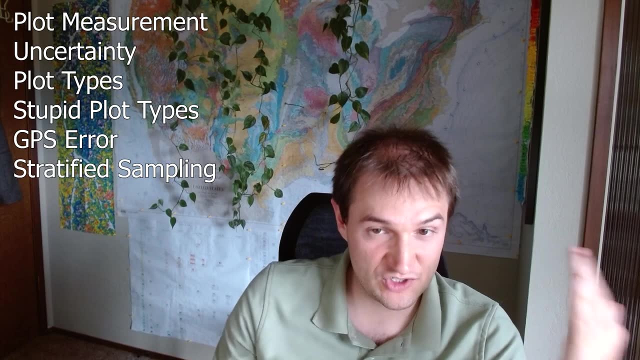 We've talked about the different types of plots: nested plots, variable radius plots, turkey foot subplots. We talked about GPS uncertainty. We've talked about forest stratification To reduce the number of plots you need. We've talked about the cost of plots. It's a lot. 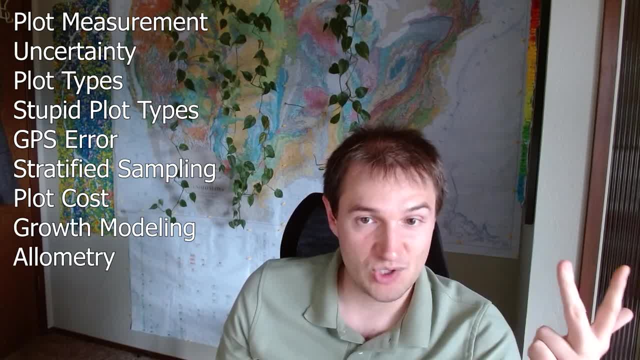 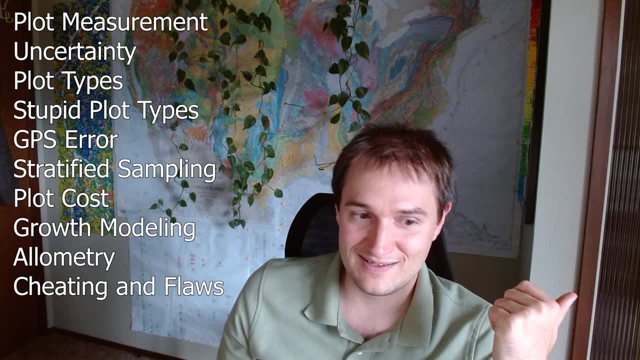 We've talked about growth and yield models, We've talked about allometry and how messed up it can often be, And we've talked about how people game the system. So that was a Whirlwind 30-minute video. Nobody's gonna watch to the end of this thing. 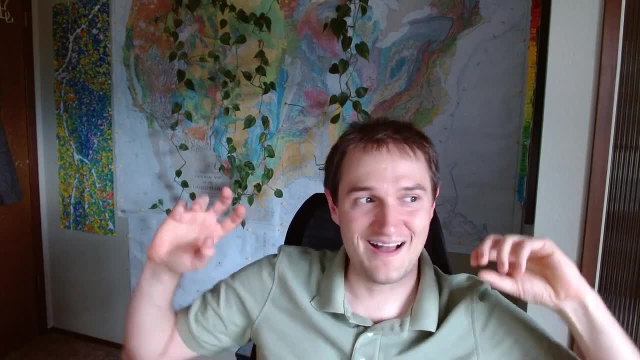 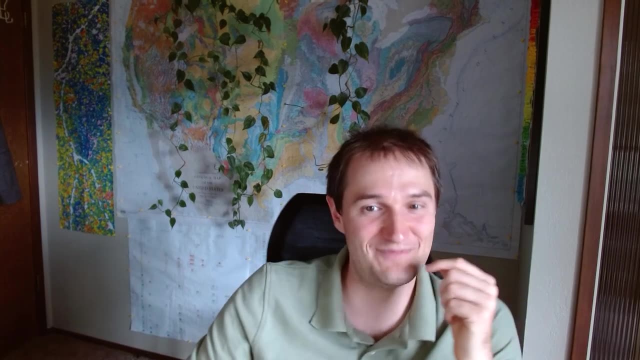 I want to put. I should put like a QR code with like a Bitcoin worth of data And if anybody actually like hits the QR code, then they get the money Right. Like, how many people are gonna do that? No, It will all come out. 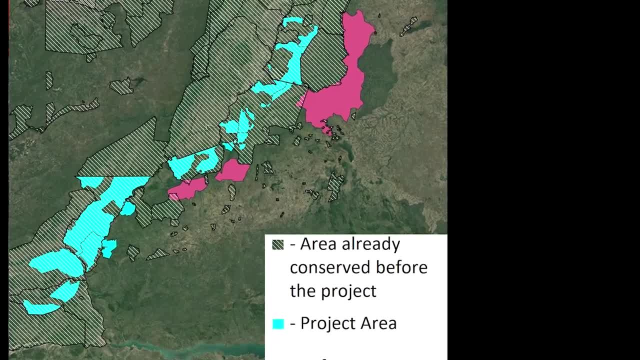 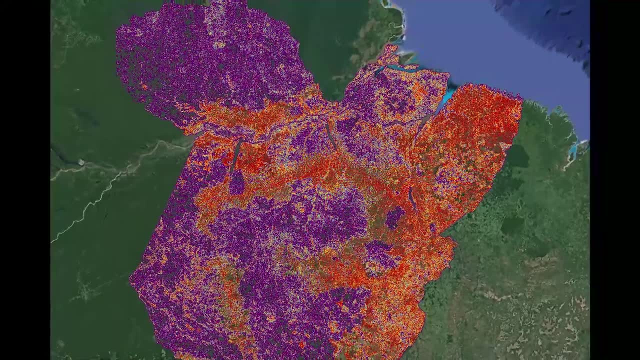 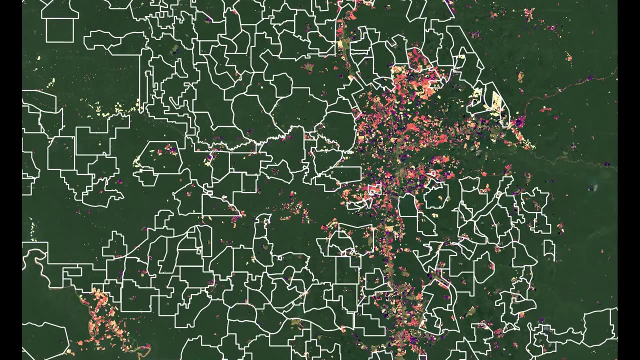 All come out in a while. It will all come out. All come out in a while. Every little stain, Every little heartbreak, No matter how messy it got, You take the Gods and the man And you throw em all in. 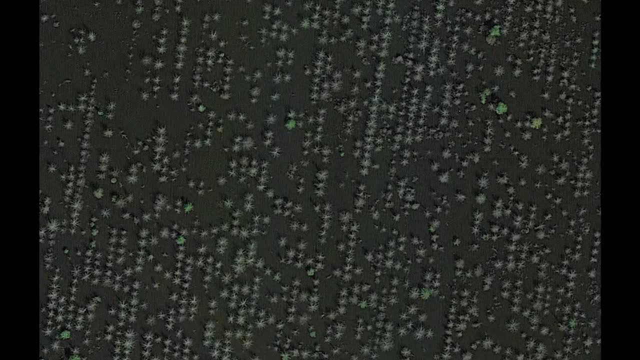 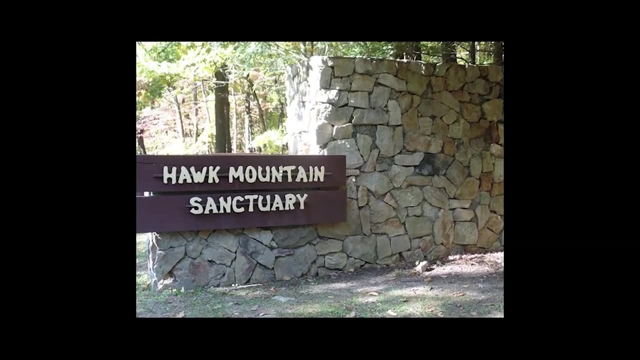 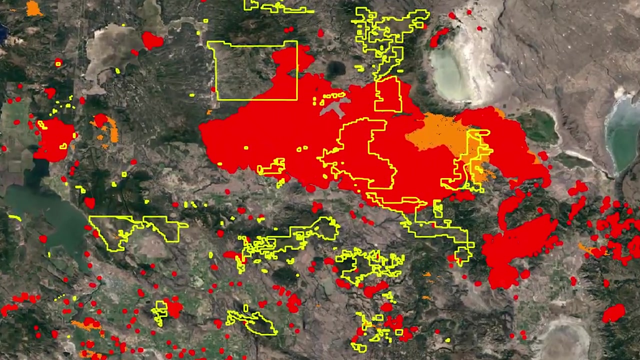 And you put that sucker on thin. Put that sucker on spin. You gotta put that sucker on spin. And the laundry list goes like this: Every tear drop, every white lie, Every dirty carpet. she let it lie and dry All the mistakes, all the wild streets. 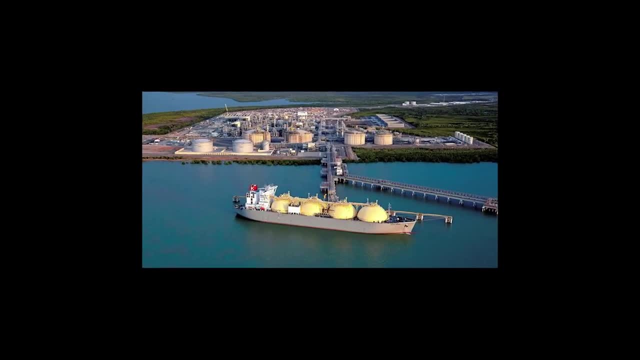 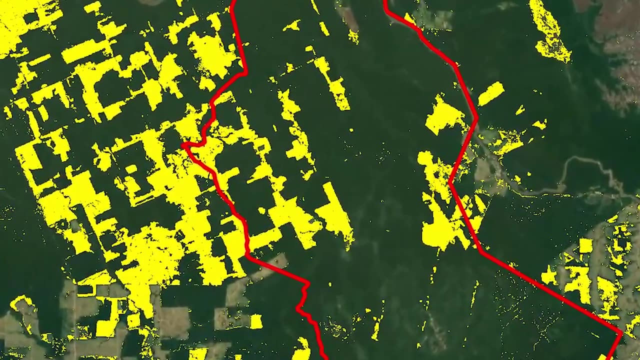 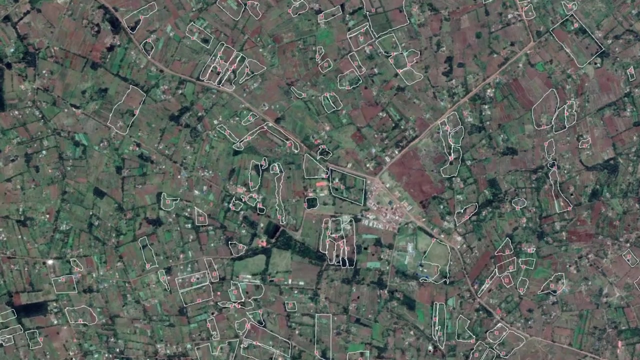 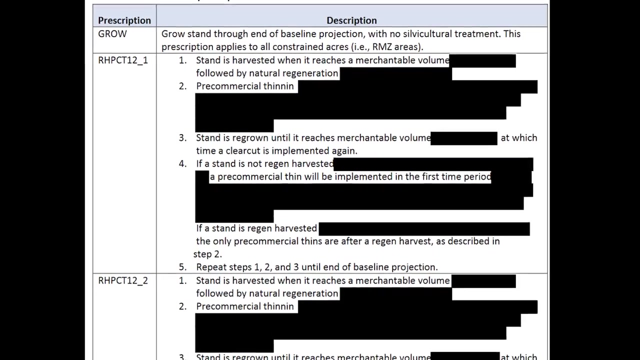 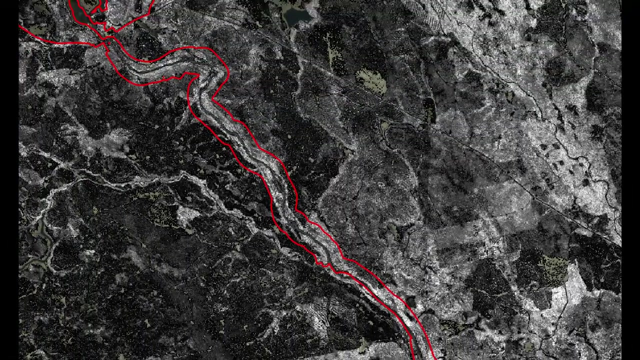 That's why the good Lord made the leash. Oh-oh, It'll all come out. all come out in a while. It'll all come out, all come out in a while. Every little stain, every little heartbreak, No matter how messy it got.